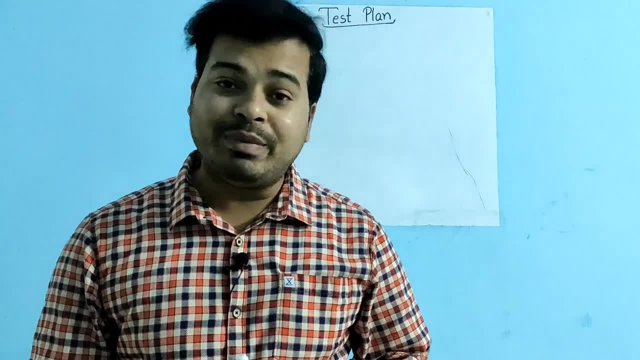 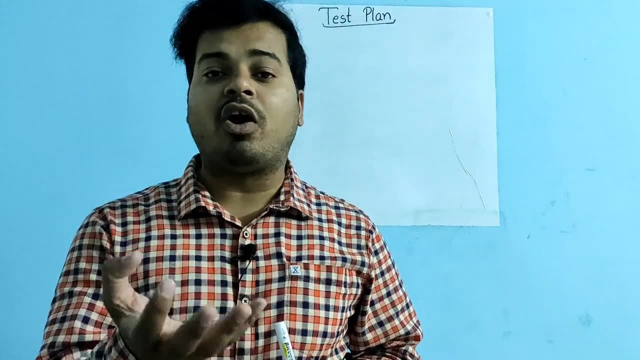 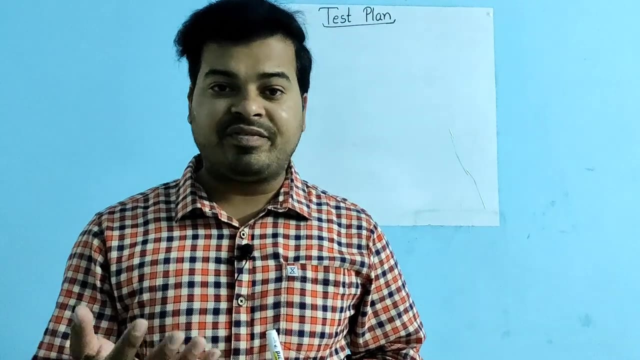 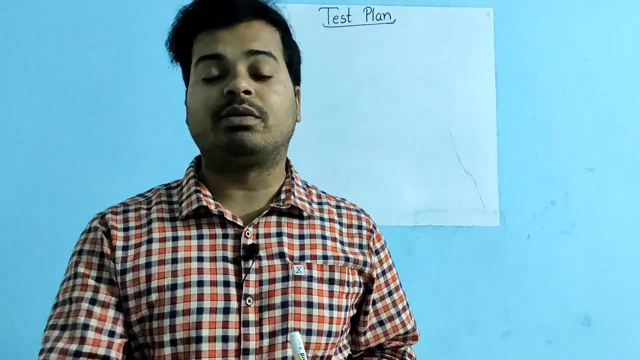 So let's get started to talk about what do you mean by test plan? So test plan is nothing, but test plan is a document which consists of all your future testing related activities. So when you are working in any company and when you are trying to start your testing process, when you are starting your testing process, before starting your testing process, there will be a test manager or test lead who will be providing you with the information. 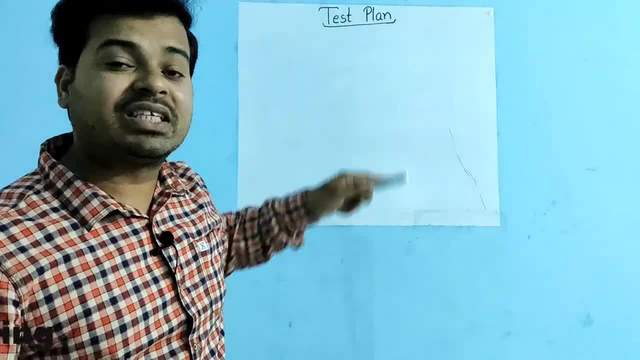 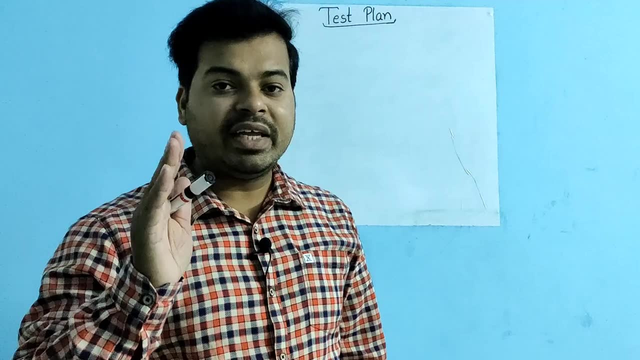 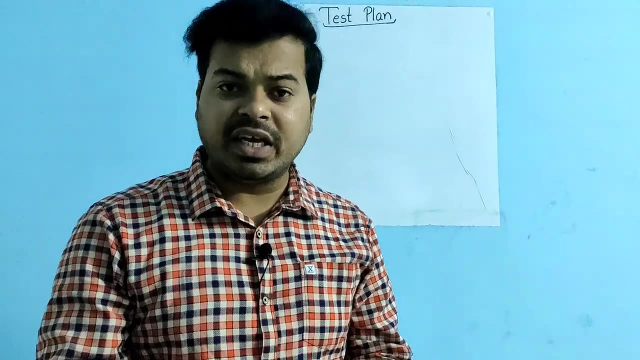 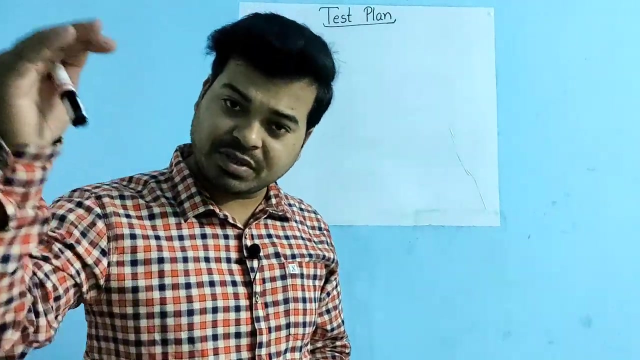 So test plan is nothing, but it is a document which consists of all future testing related activities In any company whenever they take up the project. before testers are involved in testing the application test manager or test lead or the senior most person in the team. there is no hard and fast rule that only senior person can do. anyone can do in the team, but usually test manager or test lead, anyone can do in the team. 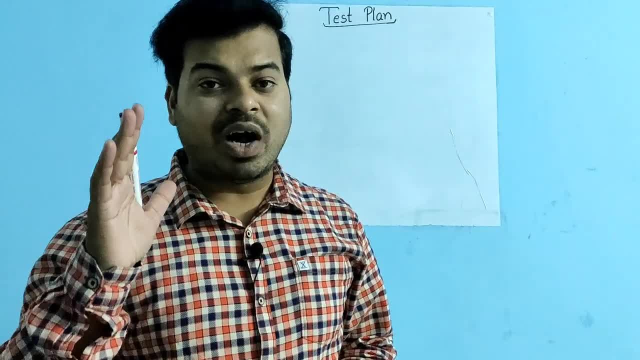 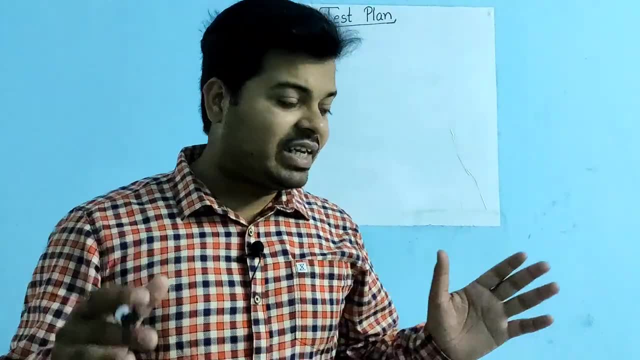 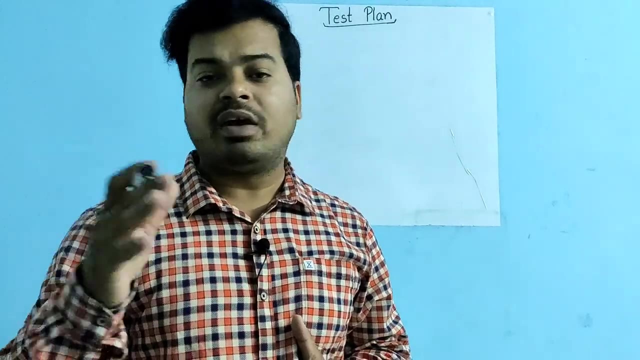 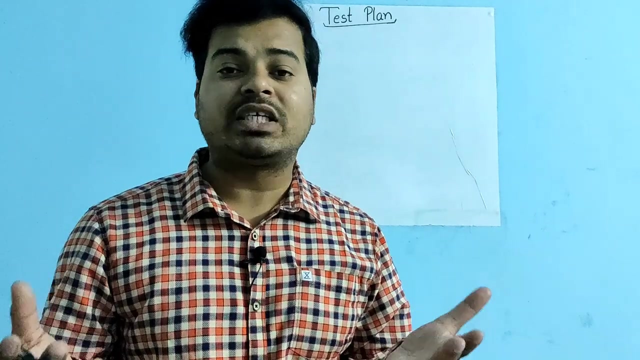 So, for example, one of them should prepare the test plan. and, guys, there is no hard and fast rule. that test plan which will look same for all the companies, There is nothing like that. But it has some standard. It has 15 attributes. This is standard. Any company will follow this if, no matter if they are product based company or a service based company. I am going to talk about in a very standard way how test plan looks like. You can follow the same in your own company. 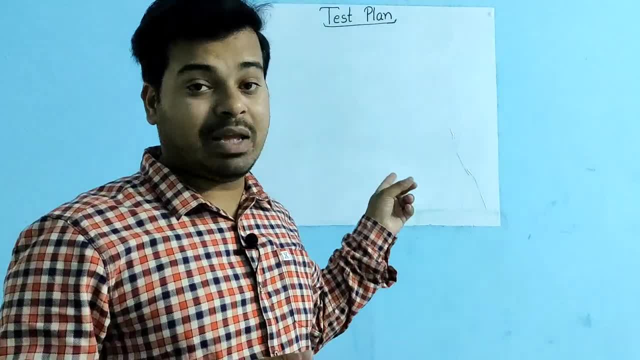 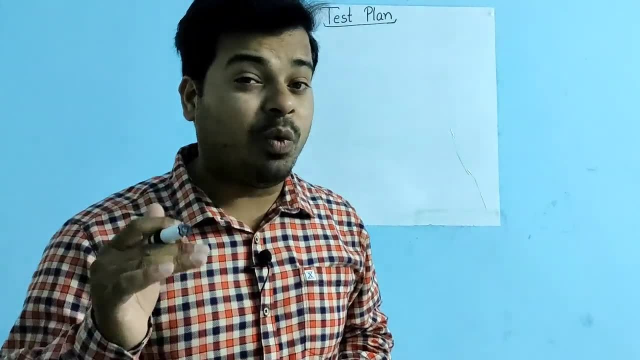 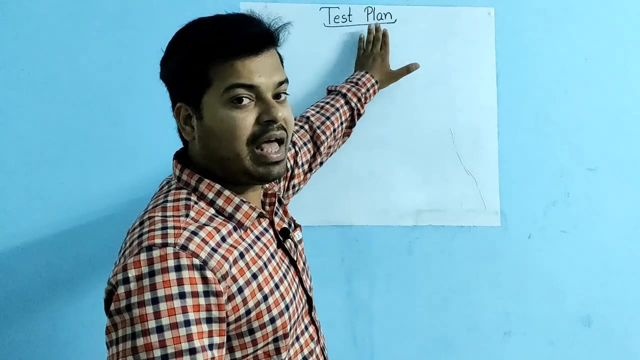 If someone is asking you interview, you can tell. tell the same. so this is what i am going to teach will be the standard. so let's get started to talk about what are the 15 attributes we have in test plan. so out of 15 attributes in test plan, the first attribute in test plan is called as objective. so under test, 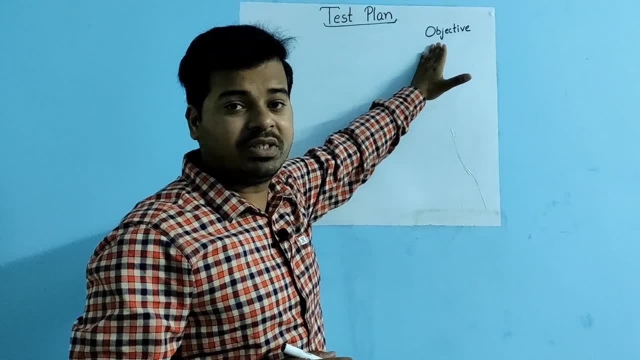 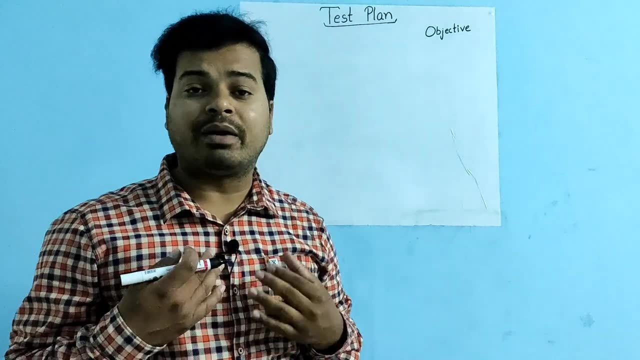 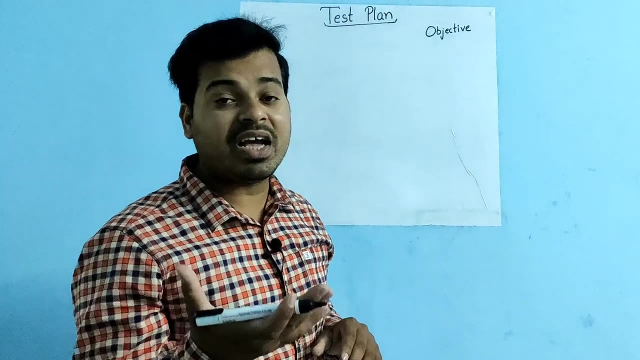 plan. the first attribute is called as my objective. under objective, we will write what is the aim of writing my test plan, why i am writing my test plan. so, in objective, they will write what, in a good process and procedure, they are going to follow in order to give the quality software. 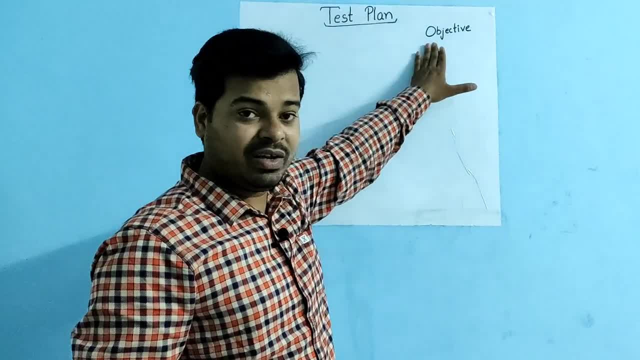 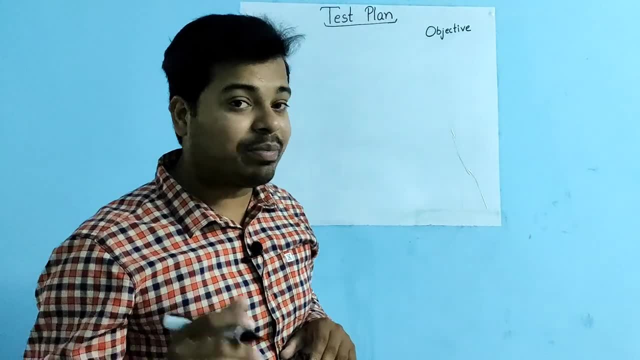 to the customer. this is the first attribute of my test plan. talking about the second attribute in my test plan is called as scope. in scope we generally write what in our feature we are going to test and what is the aim of our test plan. so in objective we will write what is the aim of our 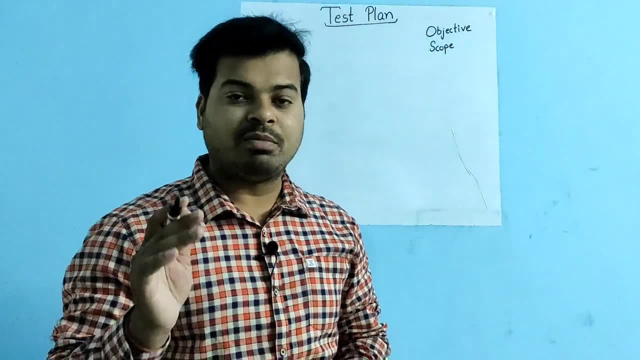 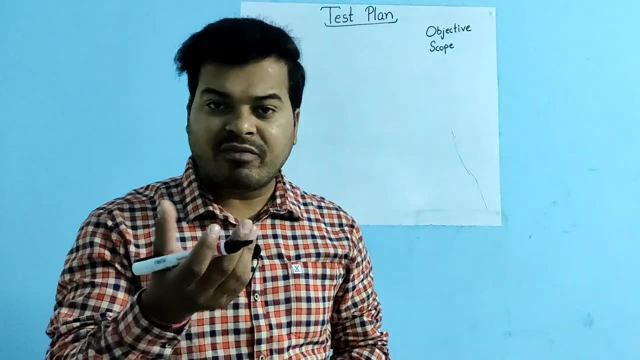 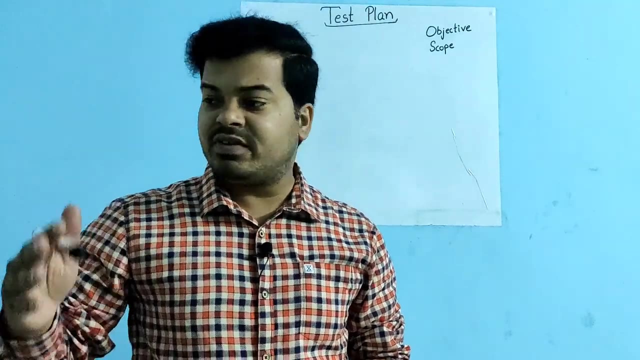 demo application. but in new test plan usually you have multiple modules, many multiple features you have. out of that, you have one, one feature which is called as about us, there is a module called as auto in which the company description is written. now, in any company about auto, still be. 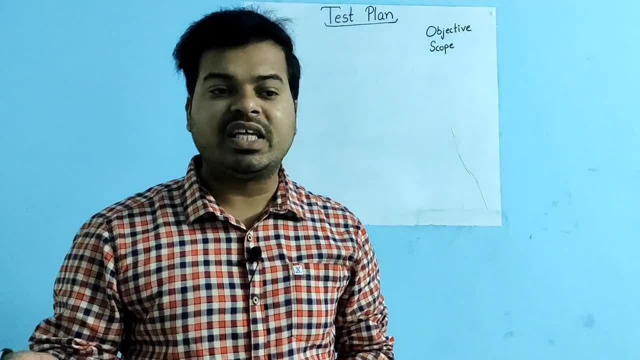 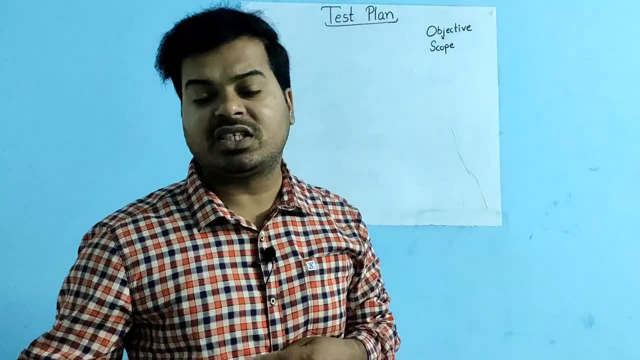 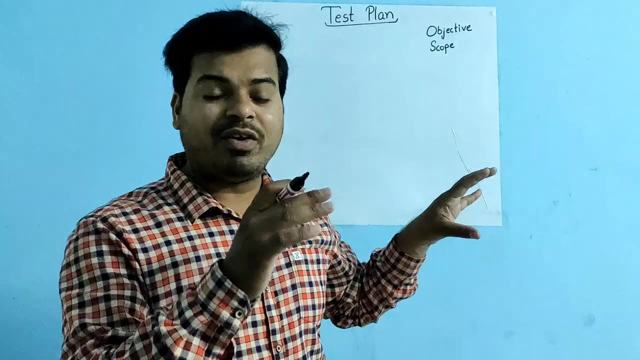 written by some technical writer. if he has written it there is no point of qa to test it again. scope: write features to be tested and feature not to be tested. suppose in my application I have 10 modules, so I will tell 9 modules I want to test it and one. 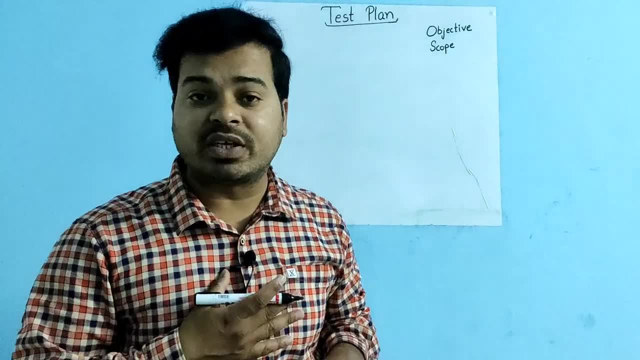 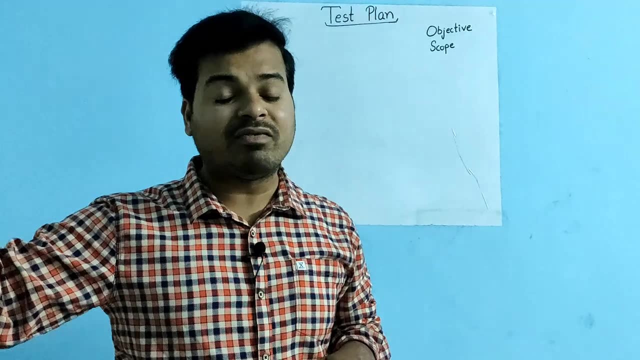 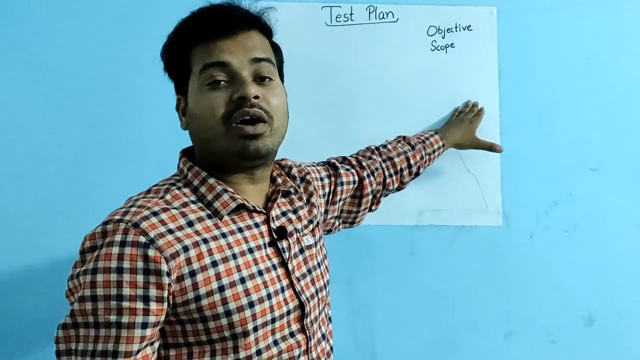 module, which is called as about us. I am NOT going to test it because it is written by my technical writer and it is reviewed by some other technical writer, so I am expecting that it is. it will work as expected. so scope, talking about the third attribute we have in test plan, is called as testing methodology. so on. 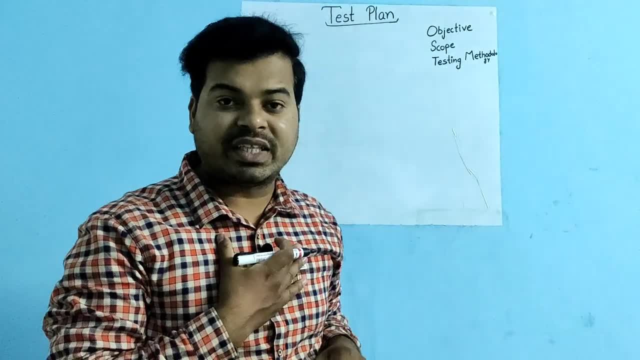 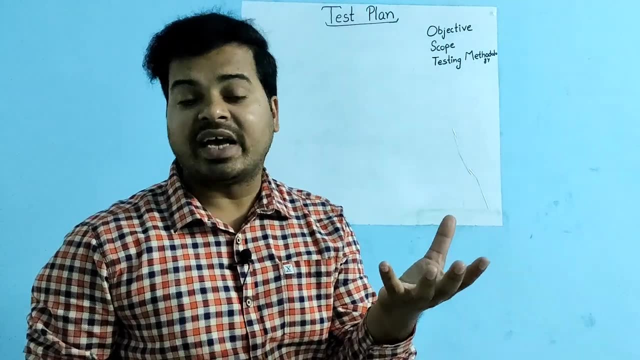 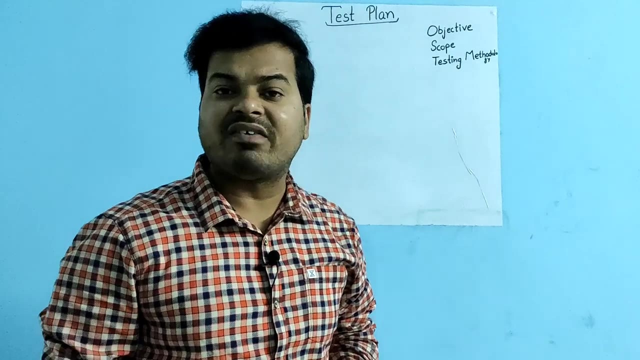 the testing methodology attribute. we have to write that, depending on our application, we have to write what another kind of testing I am going to test as a part of my testing. depending on the application, we need to select what types of testing we are going to do, let's say, if it is a web-based. 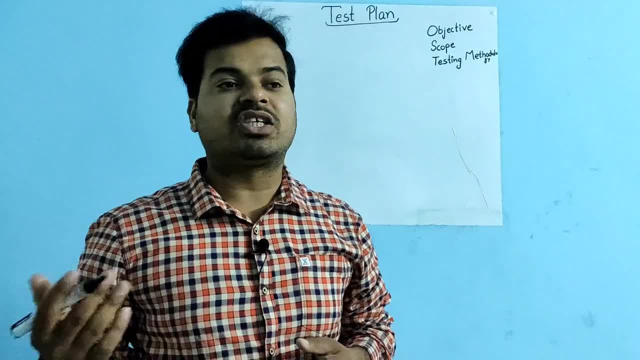 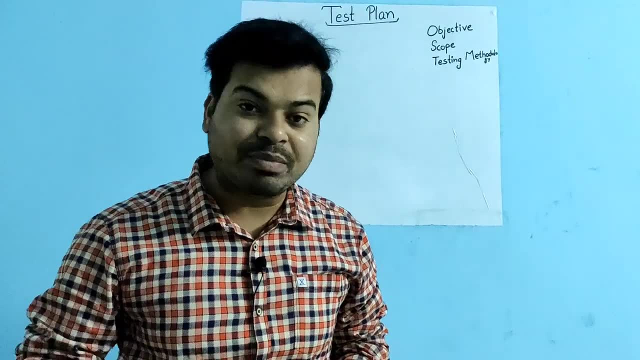 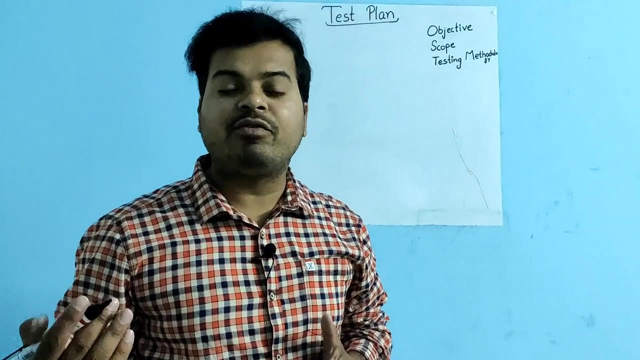 application. I will start with smoke testing, then I will start with my component testing, then I will start with my integration testing, then I will start with my system testing, then I will do my acceptance testing and also I will do performance testing for web based application let's talk about. if you have a standalone application, let's say you. 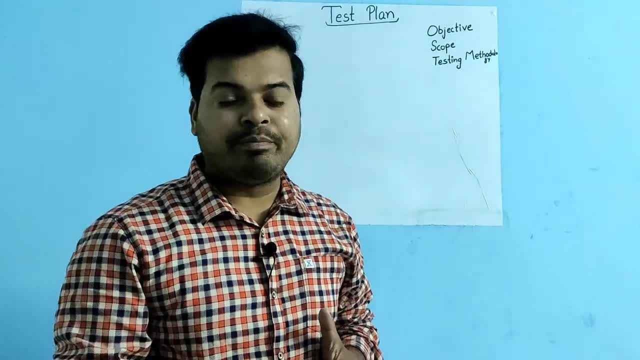 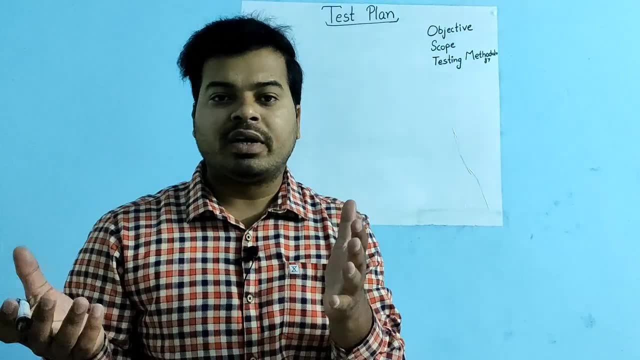 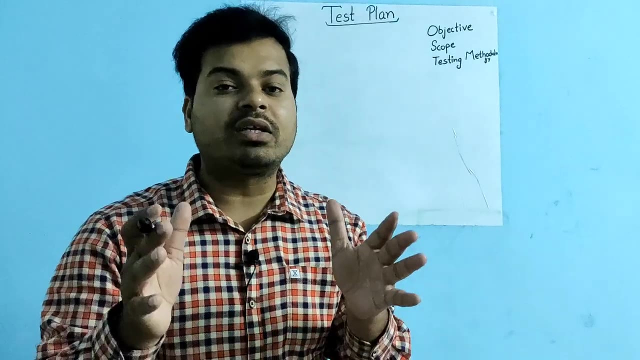 have your paint in your, in your PC paint is a standalone application which is installed in each and every individual system, so testing the performance testing on the standalone application is of no use. so that's what I'm telling. depending on the type of your application in testing methodology you 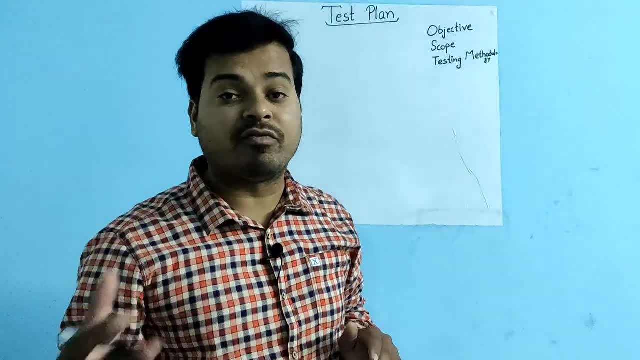 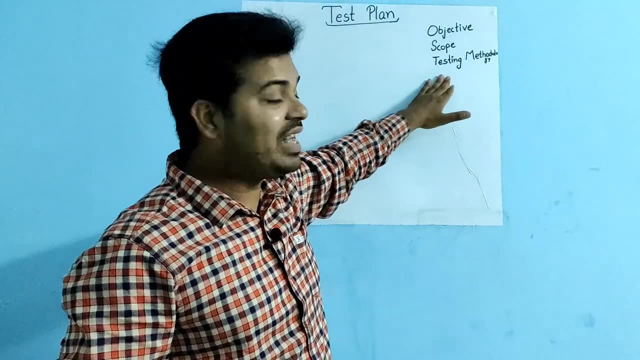 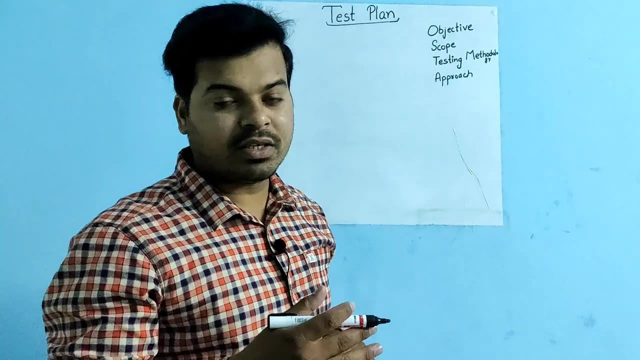 have to mention what are not kind of testing you will perform as a part of your testing. let's talk about the fourth attribute we have in test plan, which is called as approach. now, approach is something which different company will follow different things. it tells the way we go about and test. 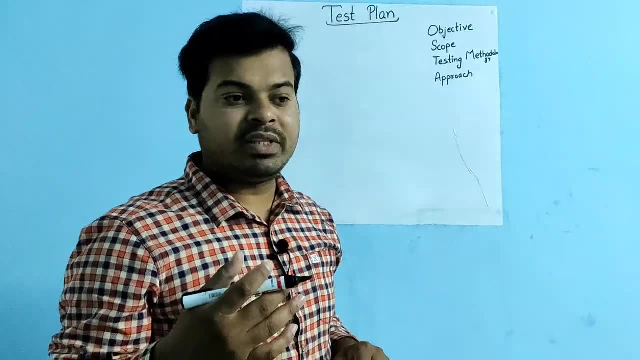 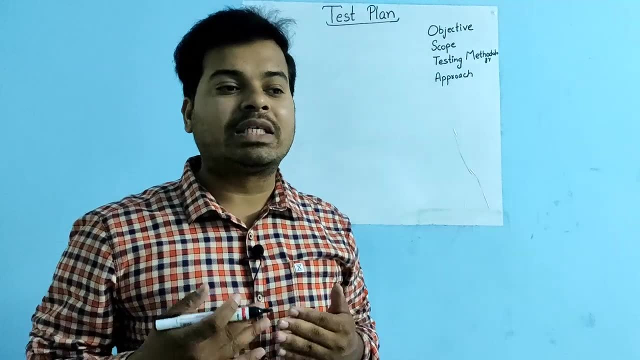 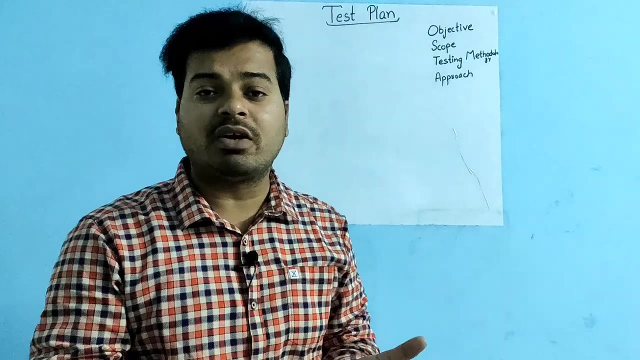 application. in future, like some companies they are, their expectation will be that their test engineer should write only test scenarios. some companies will be there who expect their test engineers to write only test cases. some company will be there who was expectation from their test engineer will be their test engineer should write both the scenario and test cases. and 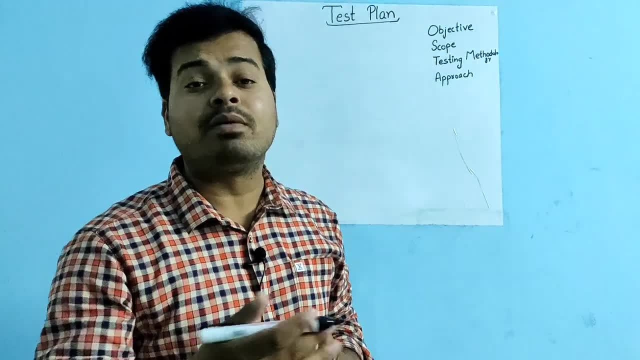 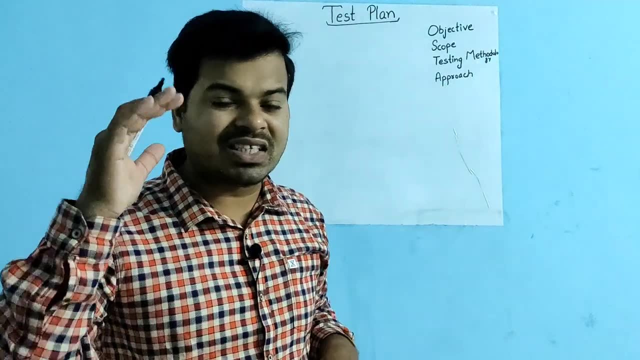 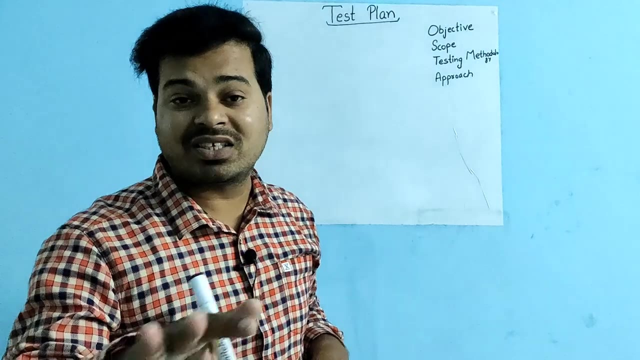 still there. there will be some companies who expect their companies to only write flowcharts. it is the way we go about and test the application future and I hope that what is the scenario, what is test cases and what is test cases and what is the scenario. I hope that is very well understandable to. 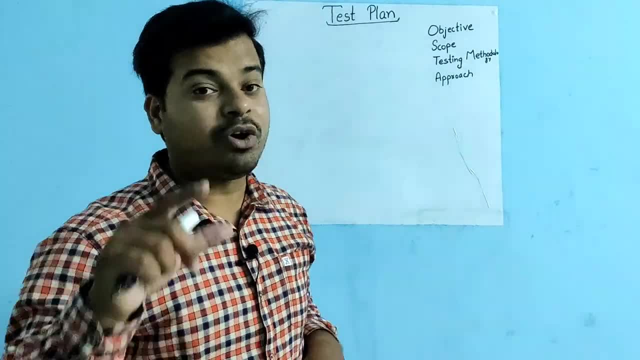 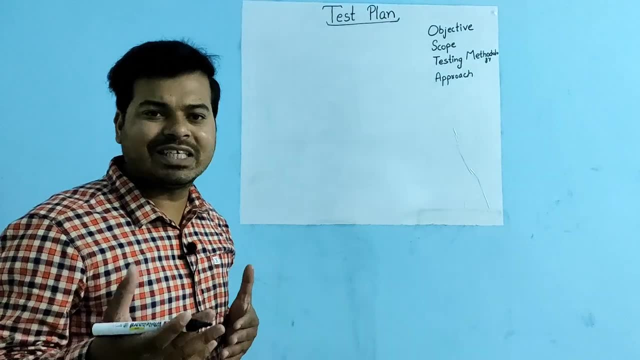 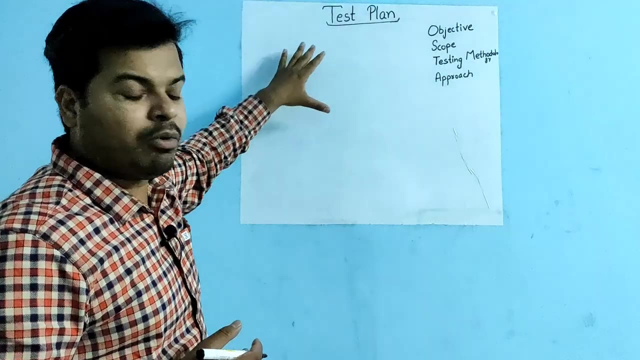 you guys. if not, link is there in the description, please watch it. talking about the flowchart, let me tell you guys what is flowchart. so some company expect you to write only flowchart. what exactly is flowchart mean? instead of writing scenarios one by one, what they will do is they will design the, all the modules. 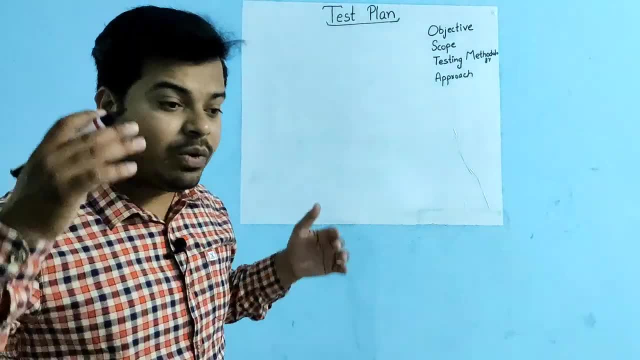 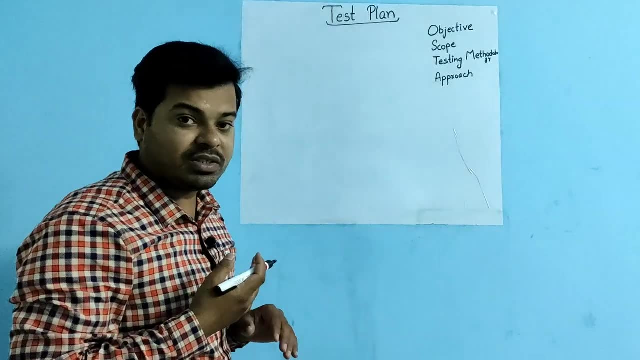 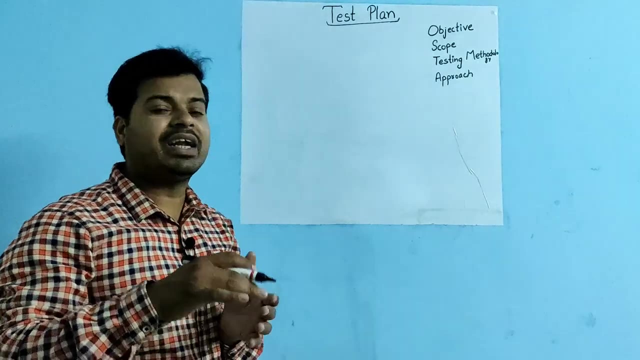 in such a way that if you look the diagram, you will only understand that which are not scenarios. you should test in order to have 100% coverage. suppose my company expectation from me is just to write flowcharts. so what I will do: instead of writing a scenario in test cases, I will just make a flowchart which 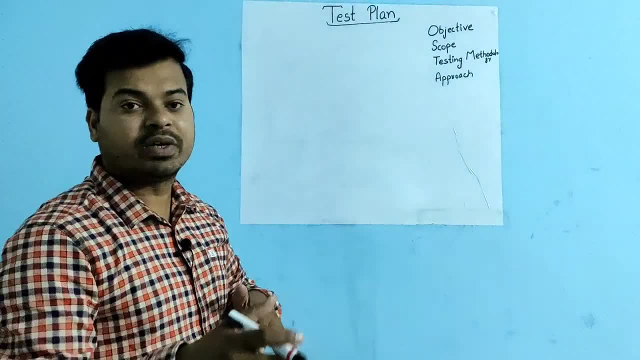 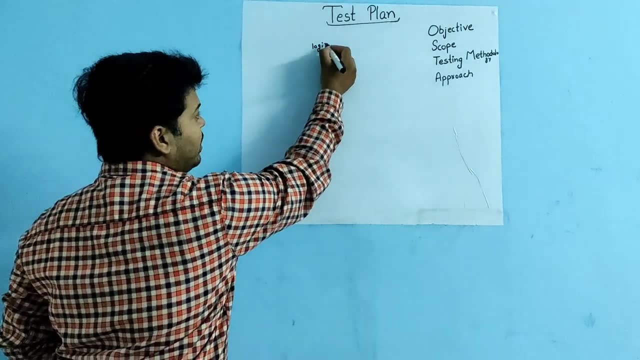 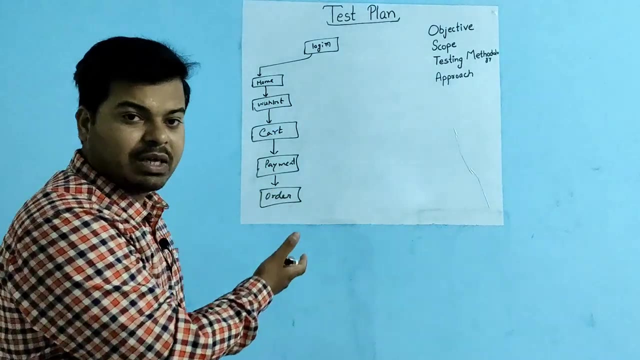 will make anyone understand what you know. scenarios are going to test it. so let's talk about a flipkart application. so I will write my flowchart in such a way that login, then home, wishlist, cart, payment order. this is just example. guys, let's say if it is a flipkart application by looking into 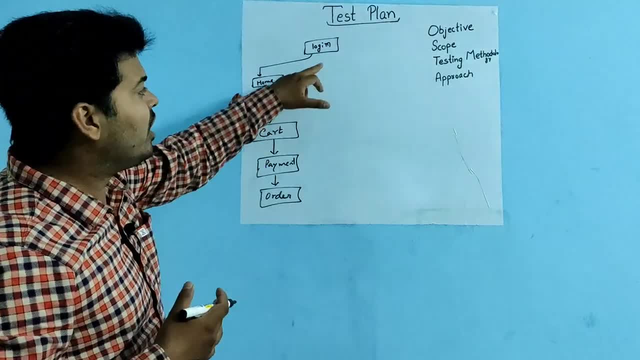 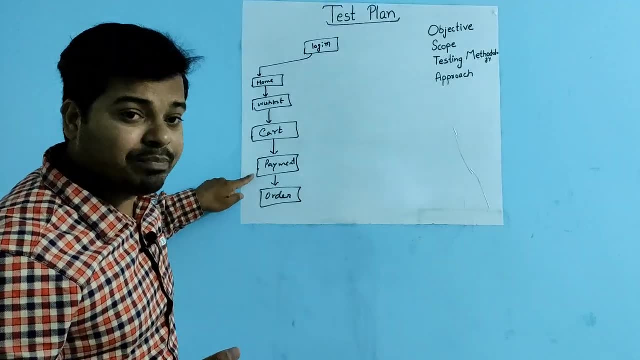 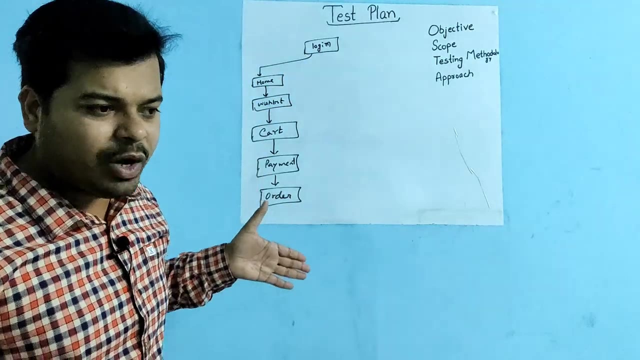 this flowchart. anyone can understand that I am just trying to tell that. login into the flipkart application, go to the home page, wishlist any product, add it to the cart, make the payment and it should be order. so instead of writing the scenario, I am just writing the flowchart, which will avoid my wastage of my 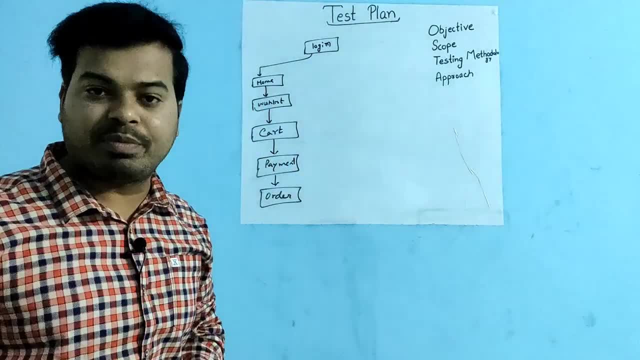 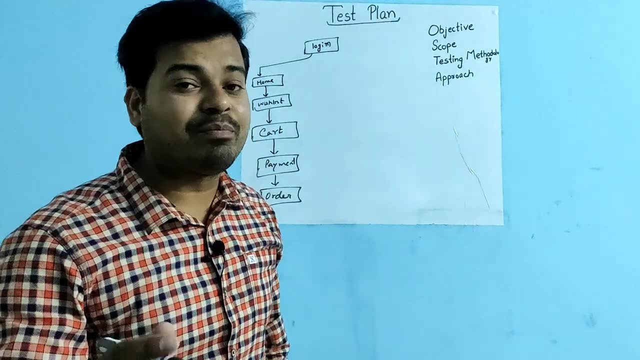 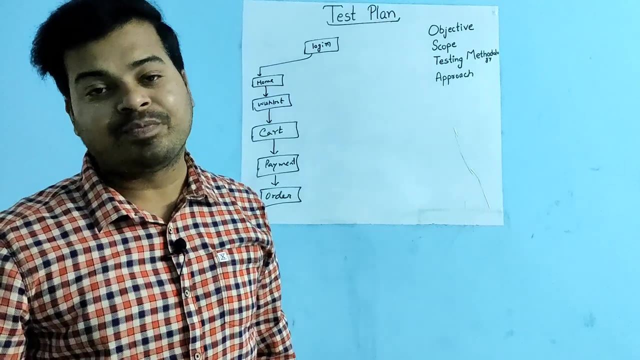 time and just by looking to the flowchart, any QA person can understand what I know: scenarios you need to cover. so approach is this approach? different company will follow different things. some company will expect their test engineers to write only test scenarios. some companies will expect only test. 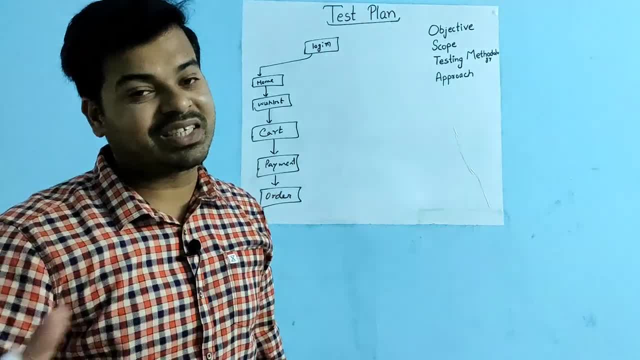 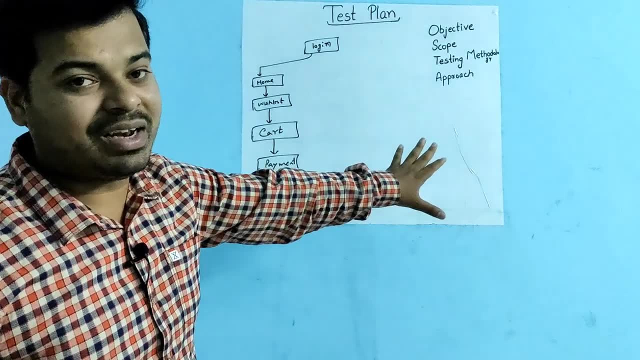 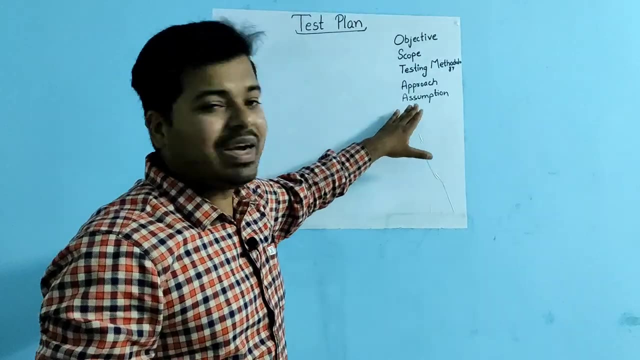 cases. some companies will expect both the scenario and test cases and some company will expect only flowchart. I hope it is understanding. well, let's move ahead to talk about the fifth attribute we have in test plan, which is called as assumptions. so while writing the test plan, certain assumption, 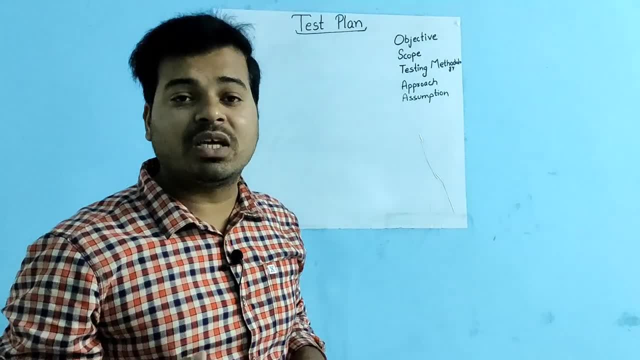 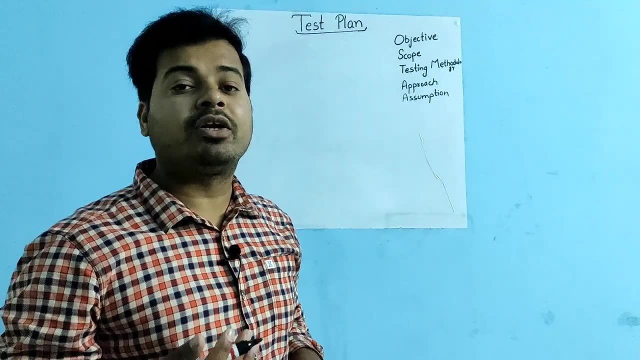 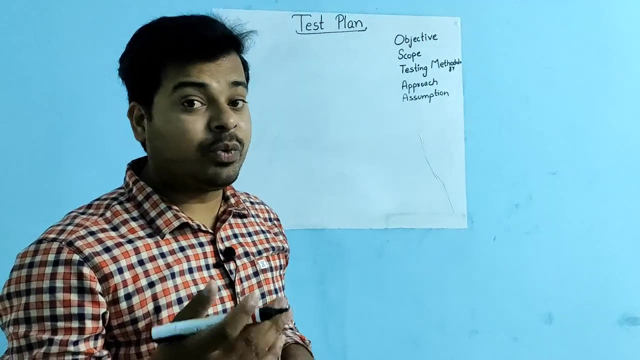 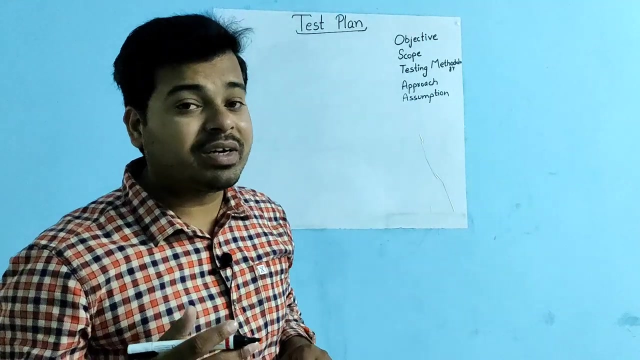 will be made. certain assumption will be made. like testers team will get proper support from the development team. this is just an example, guys. second part: like testers will get proper knowledge transfer from the development team. third part: testers will get proper document to refer the CRS, FS and all those requirements. fourth point: proper resource allocation will be. 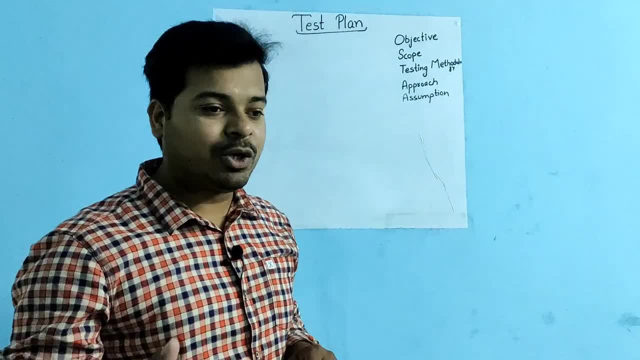 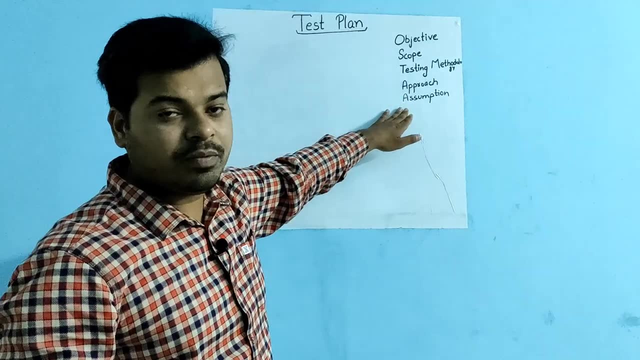 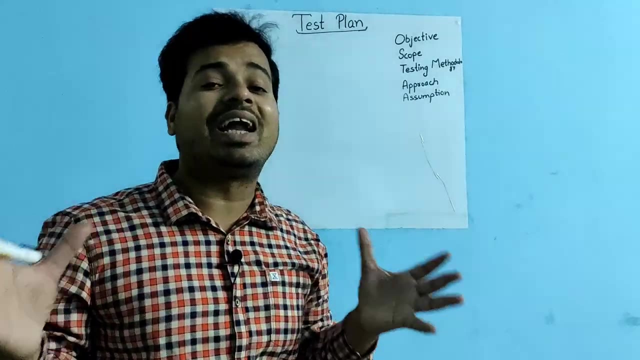 given by the company, by the human resource, to the testing department in order to complete the testing perfectly. so, under assumption, these are not, points will be there based on the company. different company will write different, different things. what are not things? I am telling it is the standard, if you. 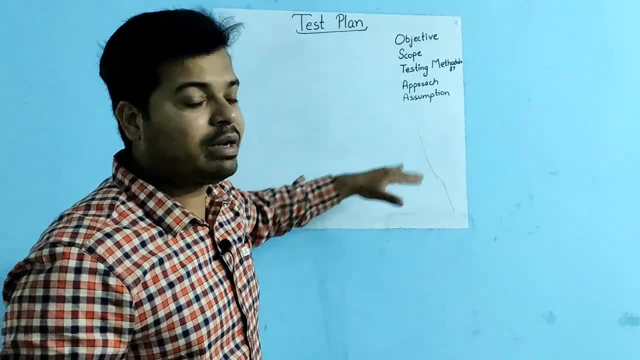 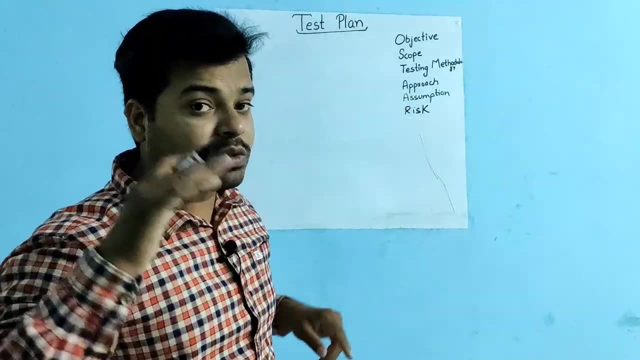 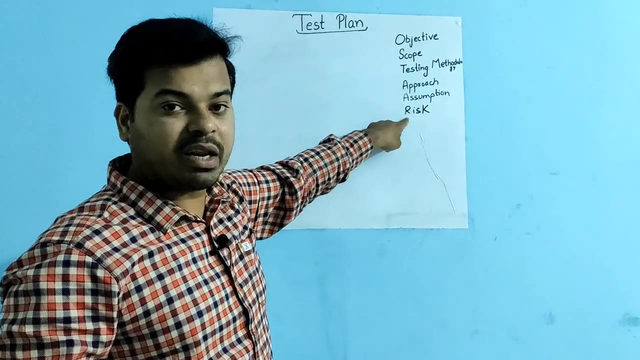 tell this to anyone, they will accept it. talking about the next attribute we have in test plan is called as risk. as I said, in the assumption those points. if anything is breaking then risk will be involved. so under risk attribute we write all the risks that can happen if any assumption is breaking. the next: 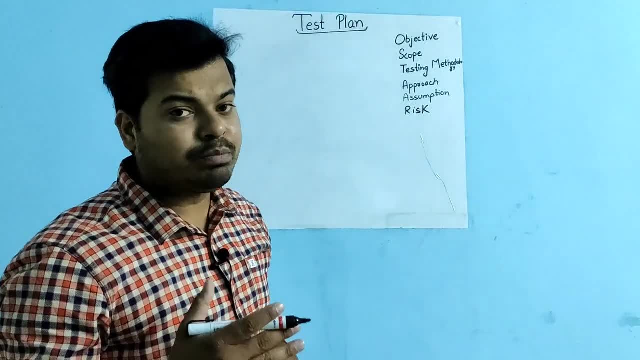 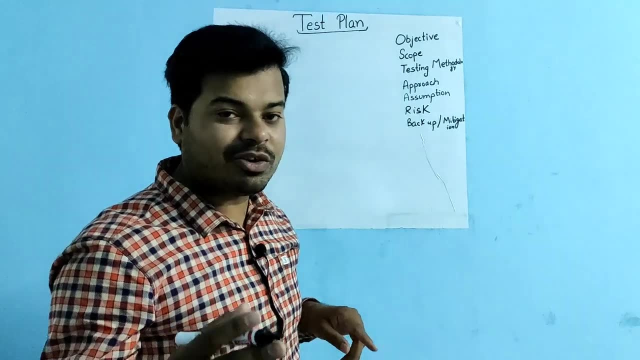 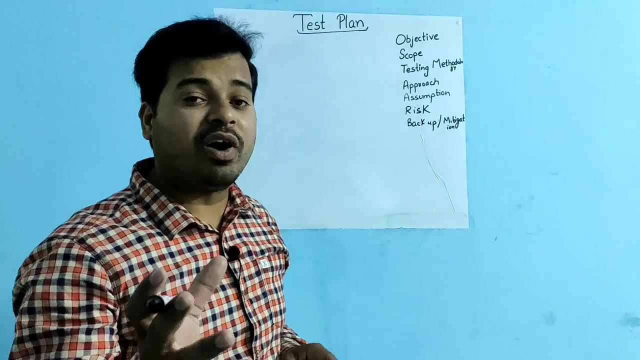 attribute we have is called as backup plan, mitigation plan. to overcome the risk, every company should have a backup plan, which is also called as mitigation plan. the purpose of my backup plan is mitigation plan is to to avoid, to overcome the percentage of mistakes: 100% to 0%. the main idea of 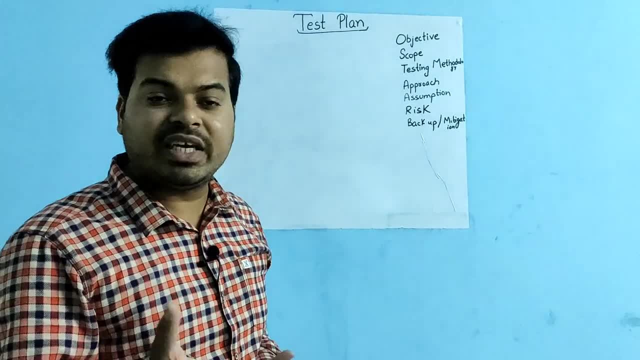 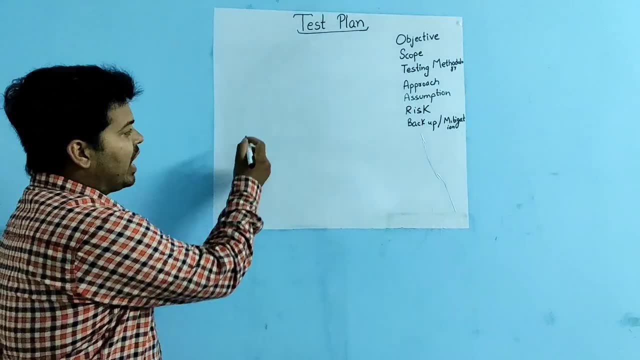 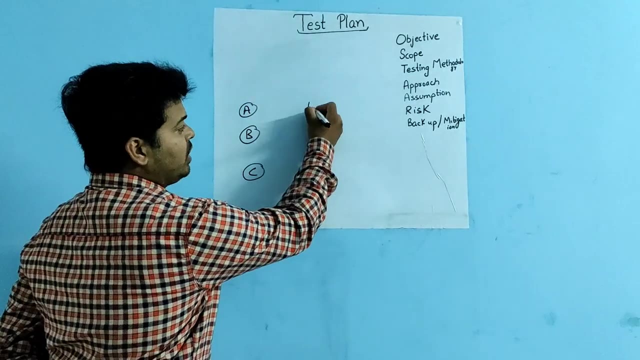 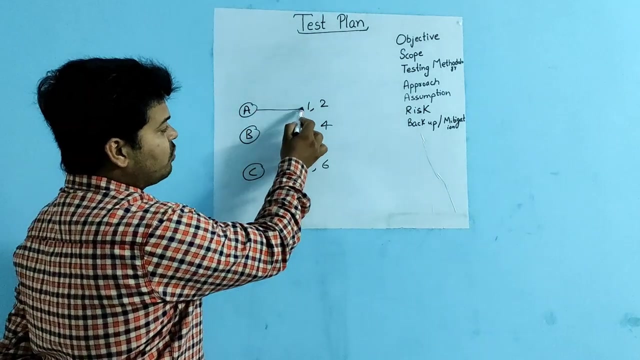 writing. the backup plan is to avoid the percentage of error, percentage of mistakes, from 100% to 0%. now let's stop. I have three test engineers- a, B and C- and I have six modules to test: test 1,, 2,, 3,, 4,, 5 and 6.. I have set this particular test engineer to focus on this. I have told. 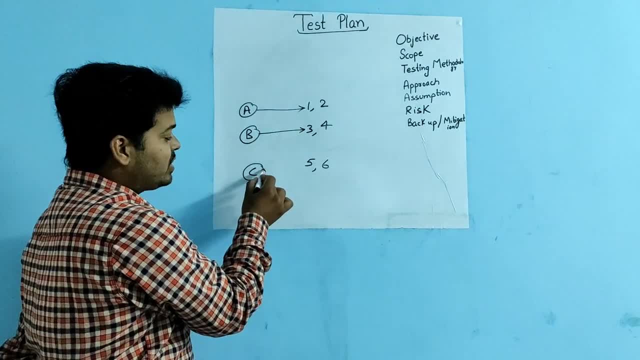 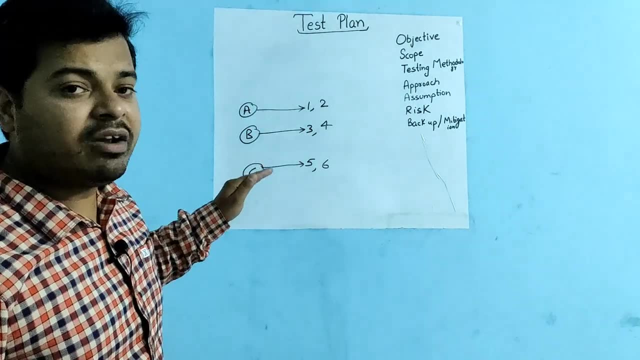 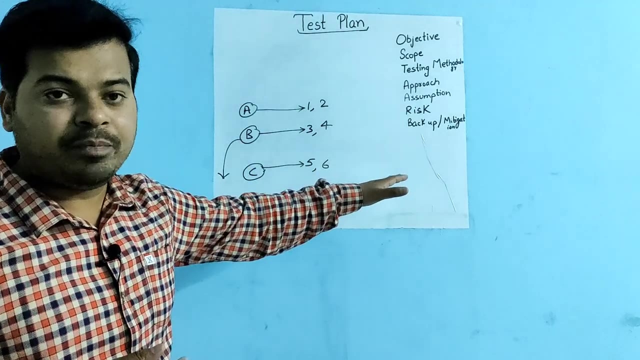 this particular test engineer to focus on this module and I have set this particular test engineer to focus on this module, 506 module. This was the plan, But in middle of some project this test engineer left the job, been working in some company as a test. 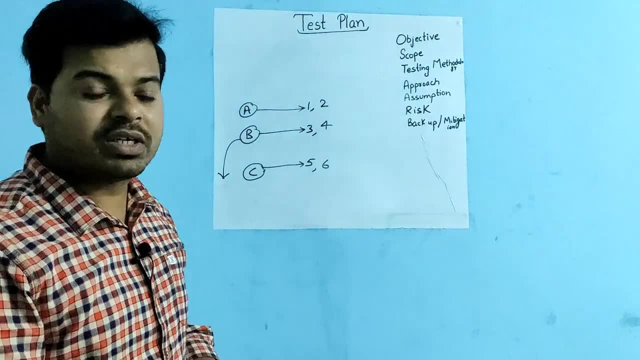 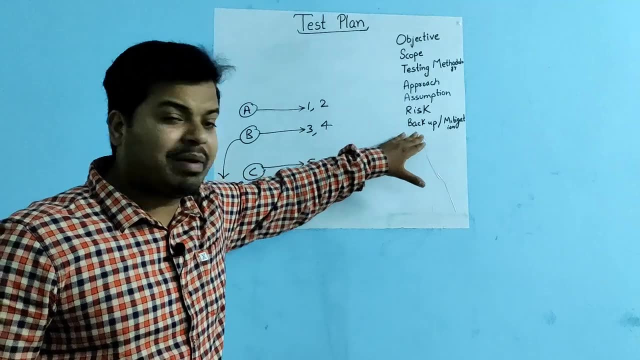 manager or test lead. I cannot tell my customer that we cannot give you the software because our team- one of the QA- has left the company. So we should have a backup plan. Now, what is a backup plan Since he has left the company? 3rd and 4th module: is there right Which? 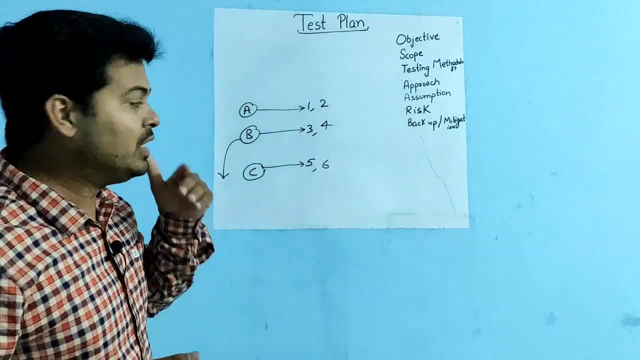 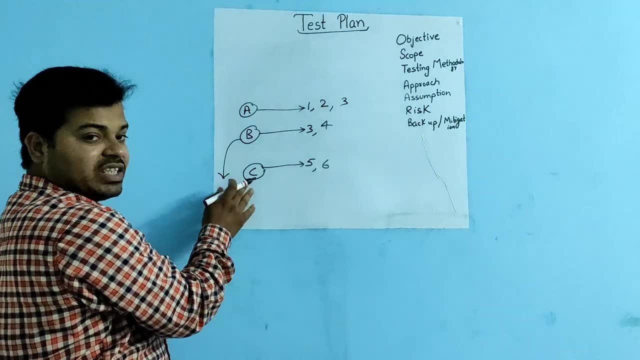 is I don't have any proper test engineer allocated for that. So what I will do is I will test my test engineer A to test module 3 and I will test my C test engineer to test the module 4.. This is the backup. 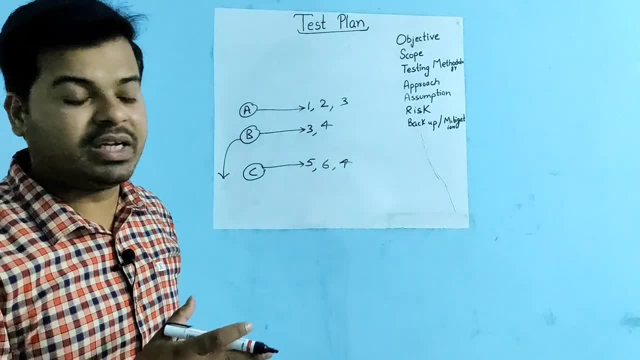 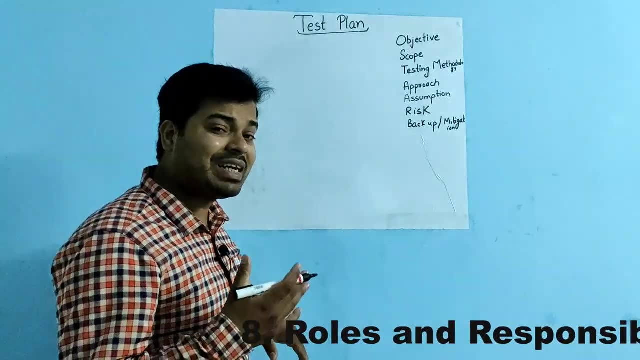 This can be anything. This varies from company to company. This is what the standard way I have explained. Talking about the next attribute we have in test plan is called as roles and responsibilities. So, under my roles and responsibility, attribute of my test plan: roles and responsibility. 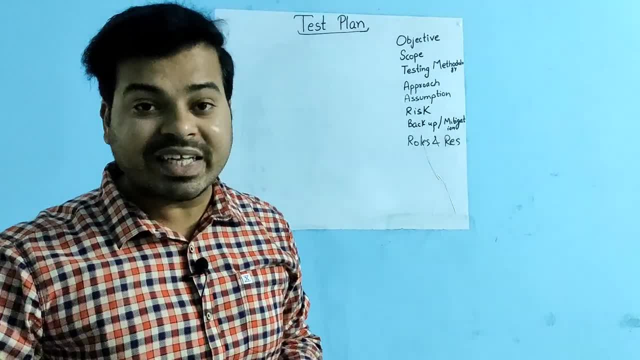 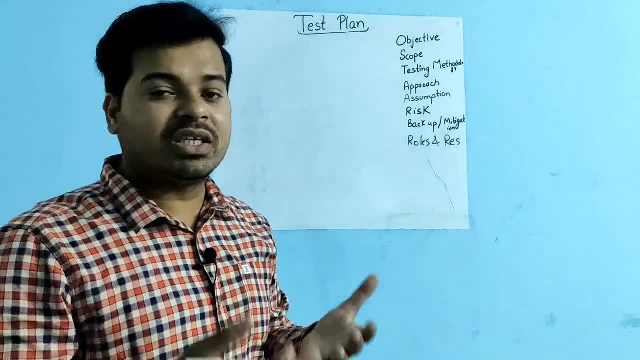 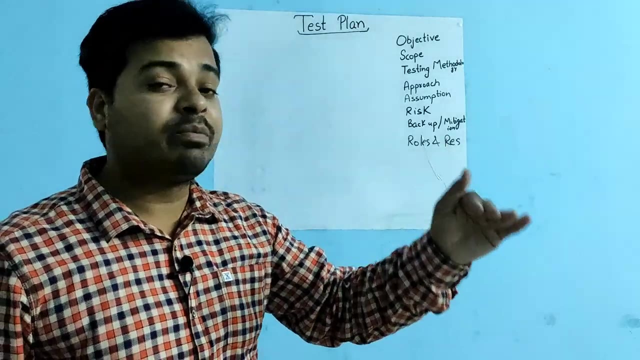 of each and every person who is involved in testing team will be written, Like. roles and responsibility of test manager will be written point to point. Roles and responsibility of test engineer will be written point to point. Let's talk. few of them, Let's see if it is. 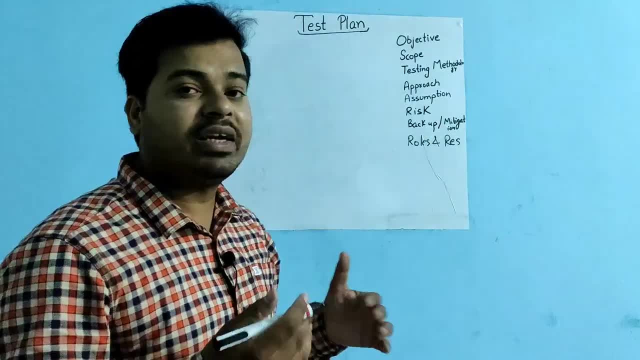 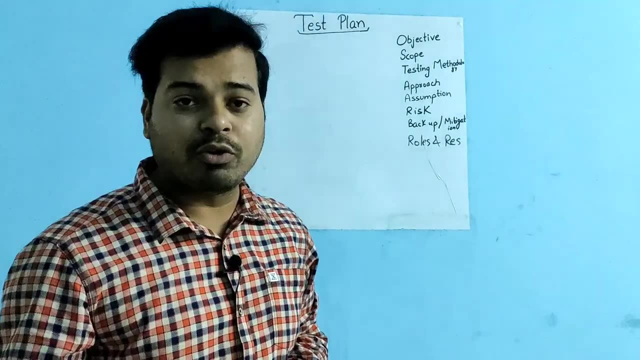 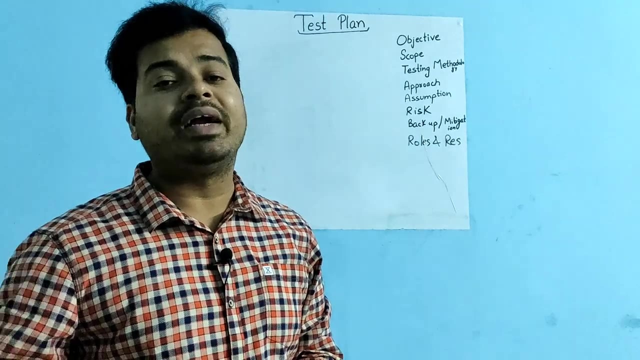 like roles and responsibility of my test manager under that tab. What are things will be there. So, talking about the roles and responsibility of my test manager, the first point will be: while testing, during the phase of my testing period, my test environment or my test bed. 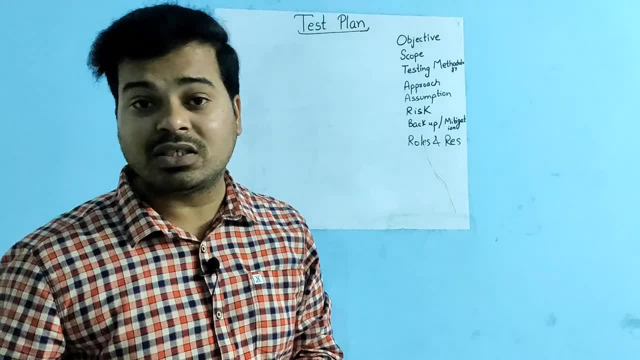 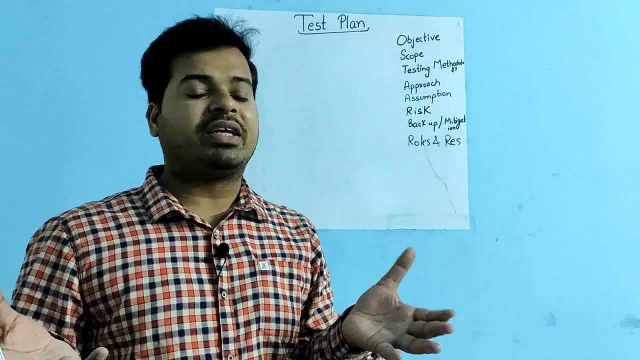 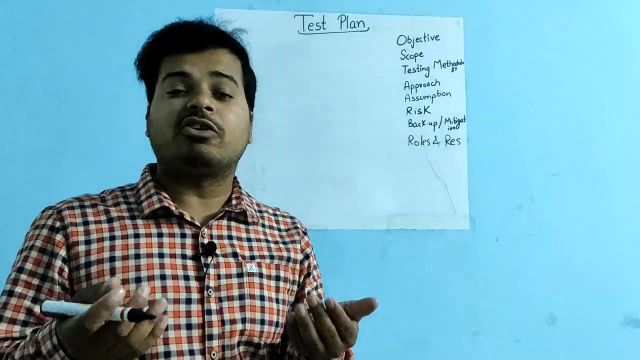 should be workable Under any circumstances means the environment where I am testing my application. that environment should work all the time that I'm testing in my QA environment. that environment should be workable all the time. If it is not workable, it is the responsibility of my test manager. 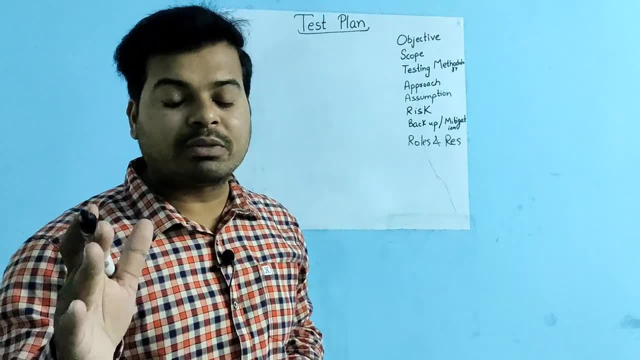 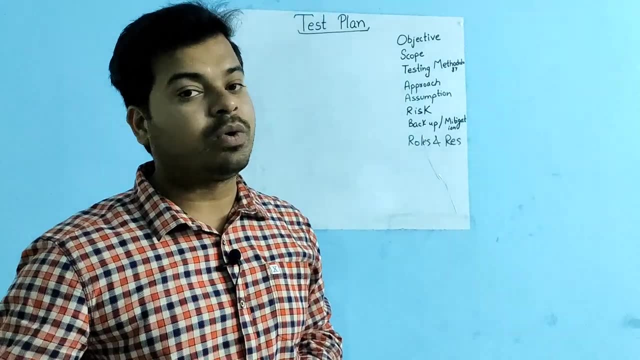 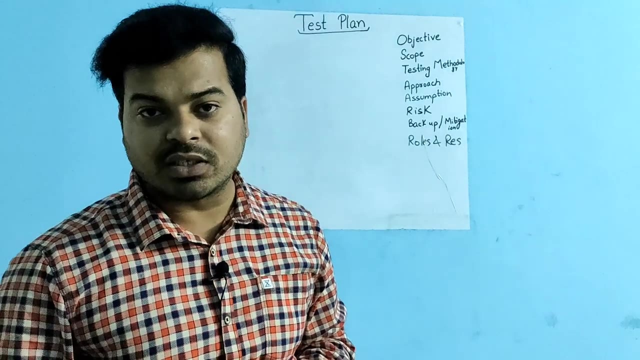 to talk with people and get it out. It will be the responsibility of my manager to communicate with customer development team and also with the shareholders, And if any Person is leaving the company, it is the responsibility of my test manager to hire the new person. 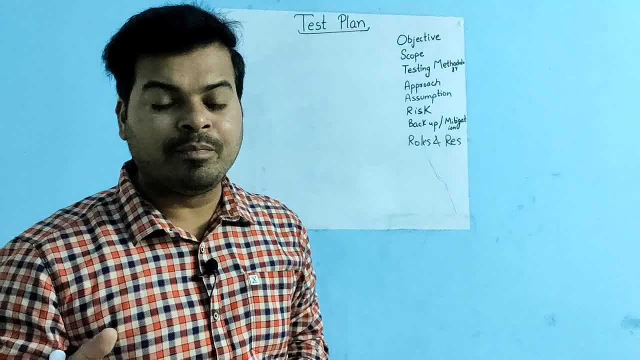 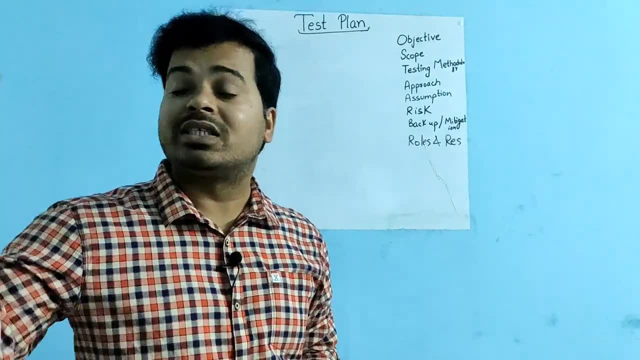 Resource allocation should be proper And, guys, whenever you join any company, test manager will be having an access to the production environment where he can see what and all things my customer are doing with my software, Being a QA, being a senior QA or test lead. 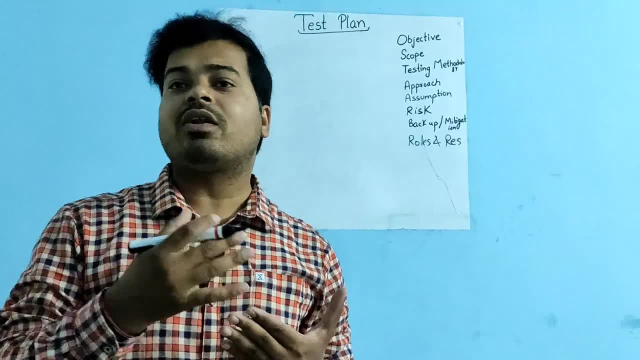 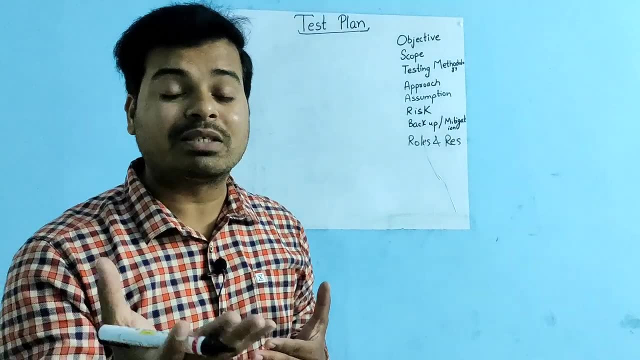 we will not be having the production environment. We cannot see what and all things, what and all scenarios my customers are doing into the production environment. So we cannot see what is happening in the production. My manager will be having test manager will be having access to the production environment where you can see each and everything- my customers 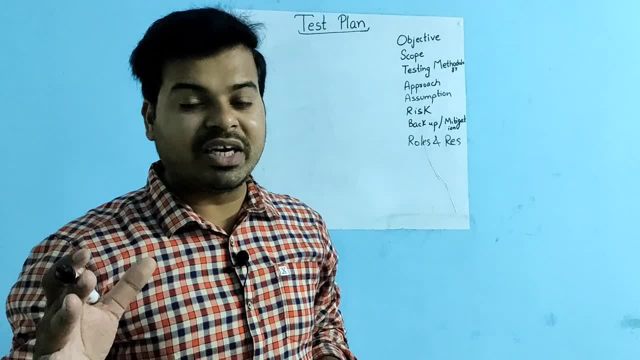 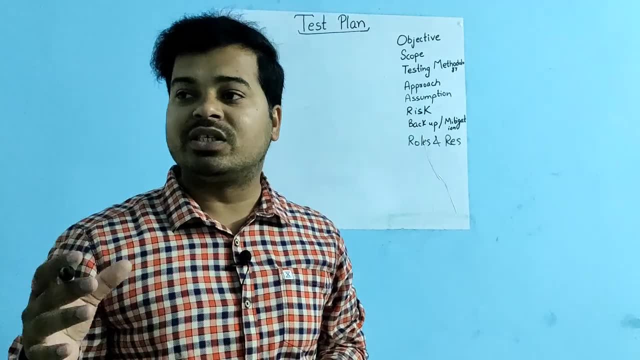 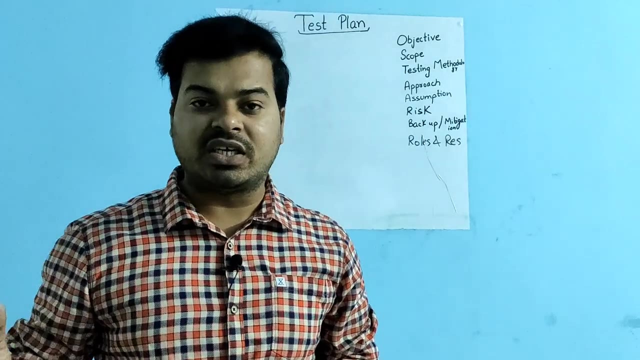 are doing. Now let's talk about the roles and responsibility of test lead. The first roles and responsibility of my test lead will be assigning modules or features to be tested by each and every individual test engineer. Assigning task to the test engineer is the. 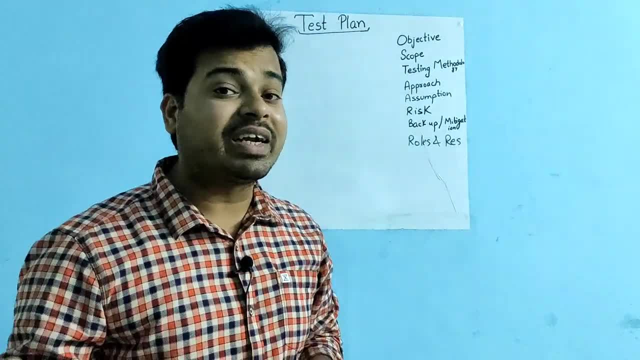 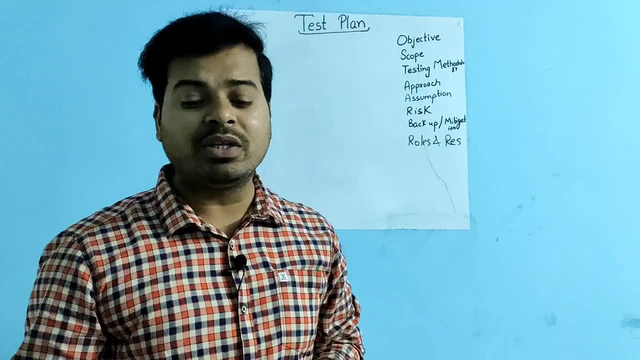 first role of my test lead: Reviewing the test case in the test case is the first role of my test lead. Reviewing the test case will be the first role of my test lead: Reviewing, approving the test cases. and if in your application there are many modules, the easy module he. 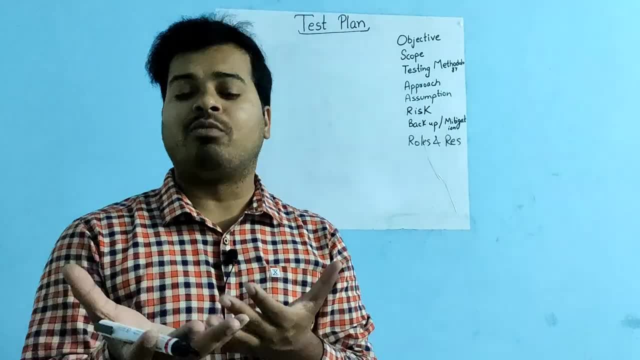 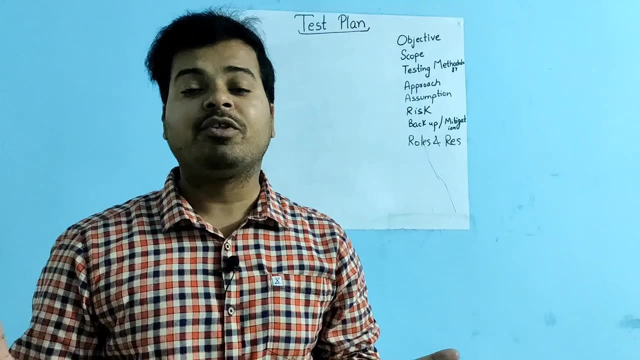 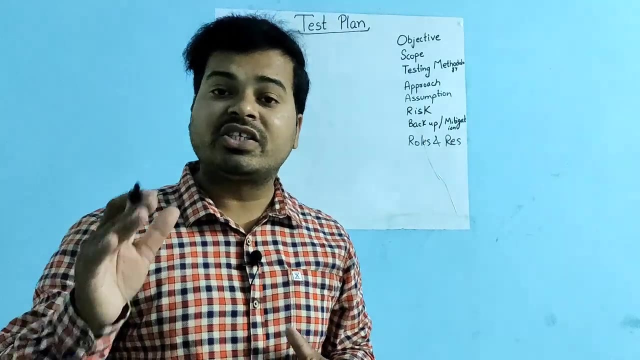 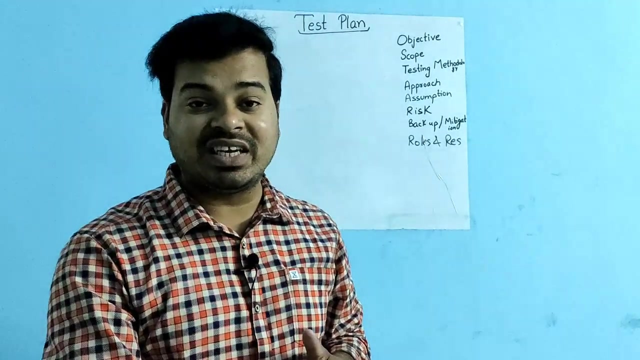 should give it to his testing team. and hard modules- the module which critical- he should take himself to test it. I mean, these are all the roles and responsibility of any test lead. talking about the roles and responsibility of test engineers are: first is understanding the requirement: writing test scenarios, writing test cases, getting it approved from your test. 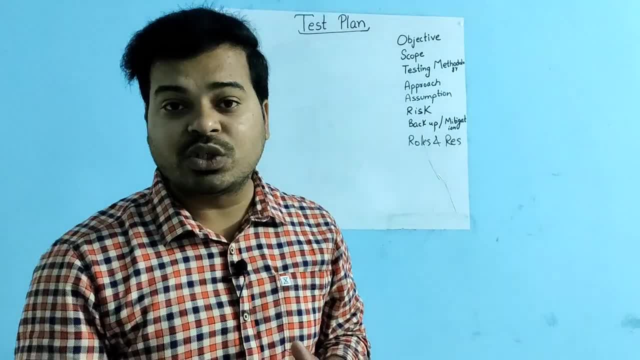 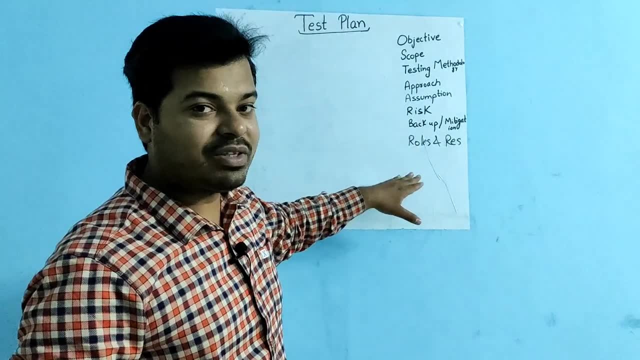 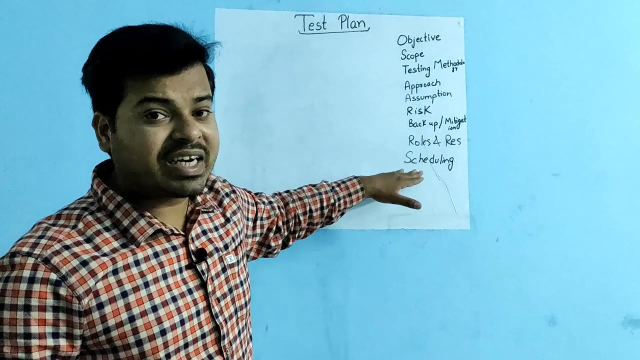 lead or your peer people, and test execution, defect tracking. these are all things comes under the roles and responsibility of my test engineers. talking about the next attribute we have in test plan is called as scheduling, so under scheduling we will write the start date and end date of each and every my testing related activity. 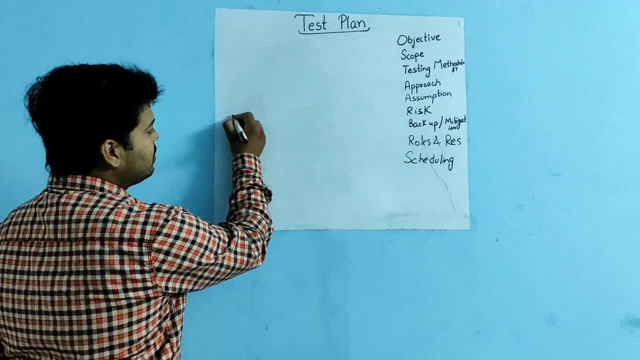 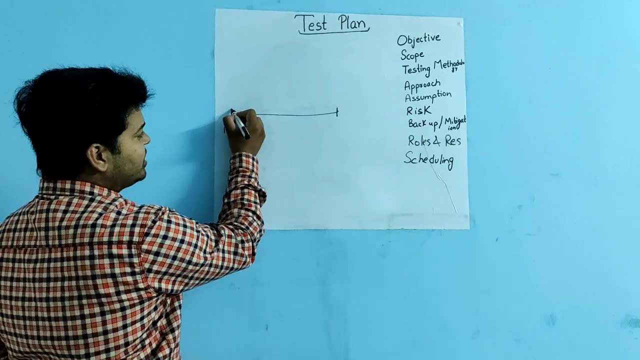 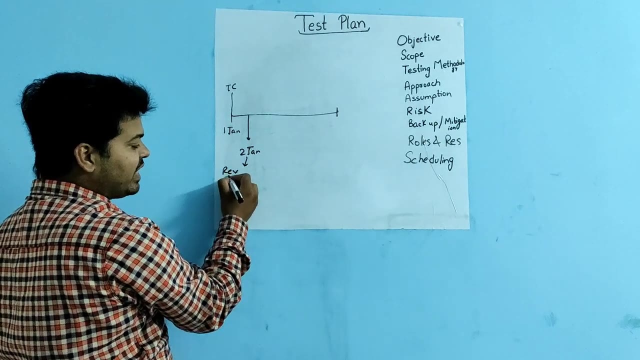 let's say whenever you are starting to test your application: this is one cycle. let's say so. this is your first jam. so, first thing, you are telling that I will write my test cases. second jam: you are telling that you will review your test cases. you will get the approval of test cases. third jam: 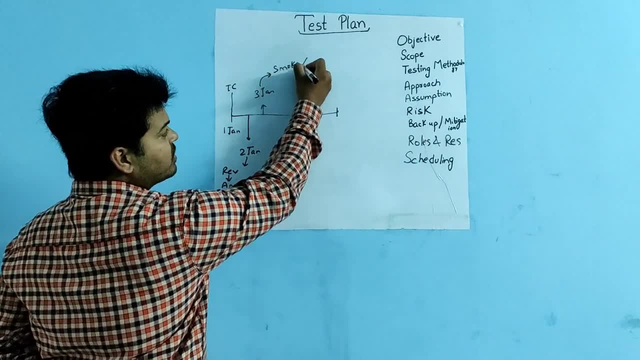 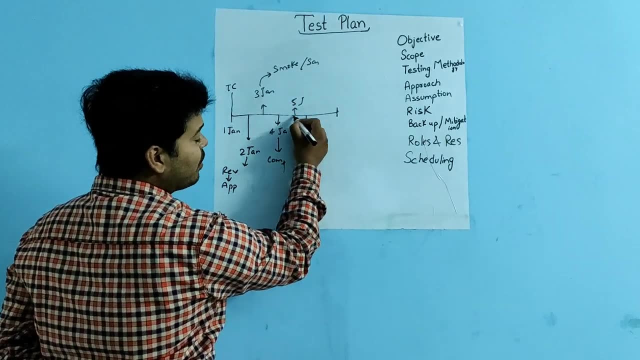 you are telling that we will do smoke testing or we will do sanity testing. fourth jam: we will do component testing. fifth jam and twelfth jam, we will do the test test and the third jam we will do single test test. and sixth Jam, both the day, we will do integration testing, each and every testing. 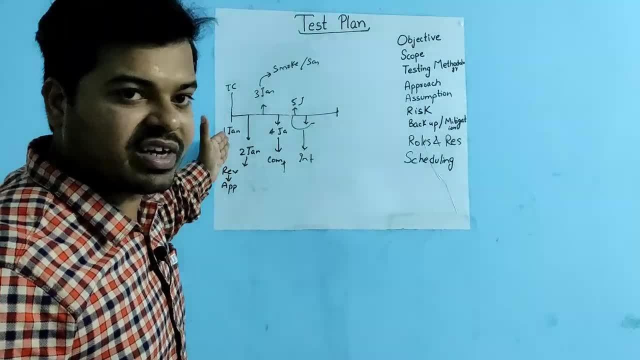 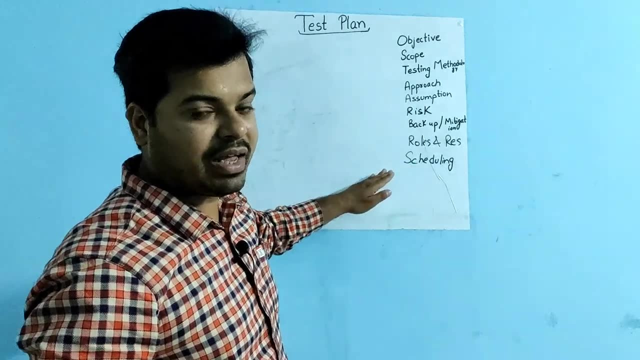 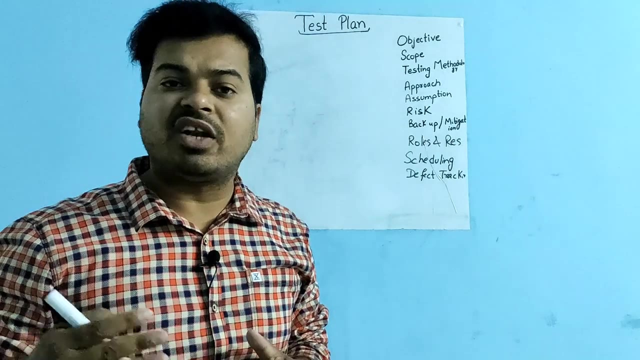 activities. what you know you are going to do, the starting day of it and the ending day of it, you gonna write it in your scheduling. the next attribute we have in test plan is called as defect tracking. when you are testing the application and you are getting some defect, you will log into the defect. 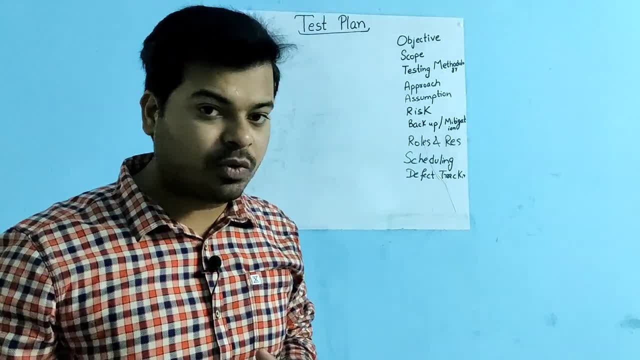 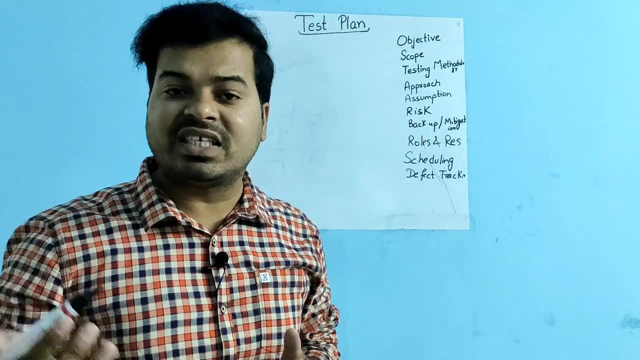 tracking tool, let's say Jira or bugzilla a tool. whichever company is following, you will open it. log the bug. you will log the bug. then developer should fix it. whenever he is giving a fix, you should retest it. if it is working, fine. you will either close the bug and if it is not working, 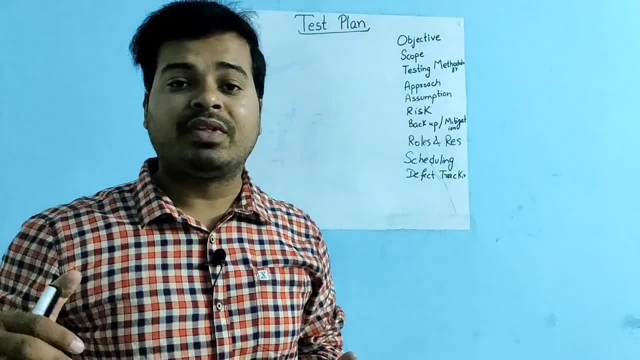 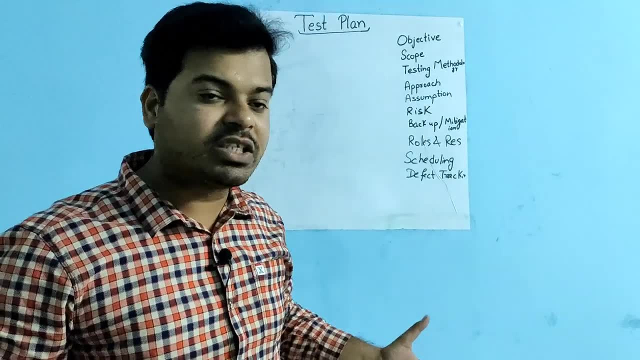 you will reassign the bug again to the developer. so this whole process is called as defect tracking. so under defect tracking there will be multiple components in it which they will write in the test plan, different components in the sense they can write which defect tracking tool we are using. 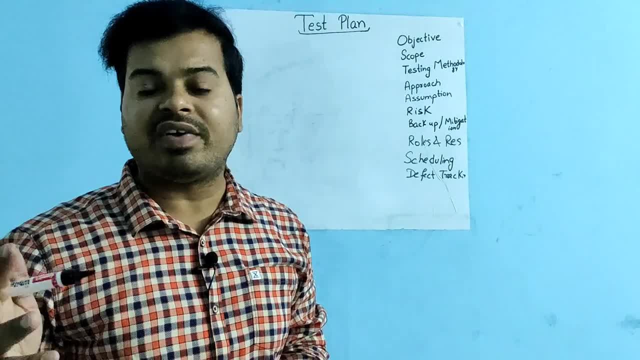 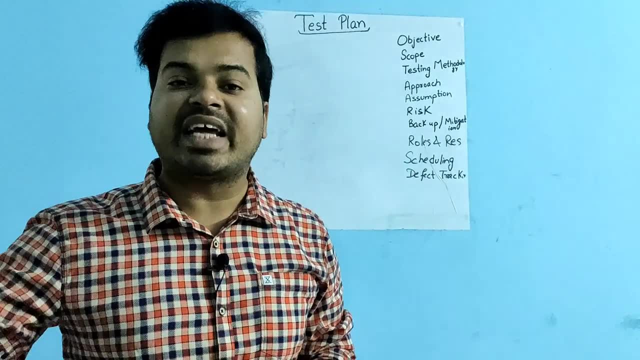 so they have to mention the name. what is the procedure to track the defect? so they have to write the procedure. what is the procedure they are going to follow while raising any bug? they will tell what is the severity types. we are going to follow, like we are following blocker critical. 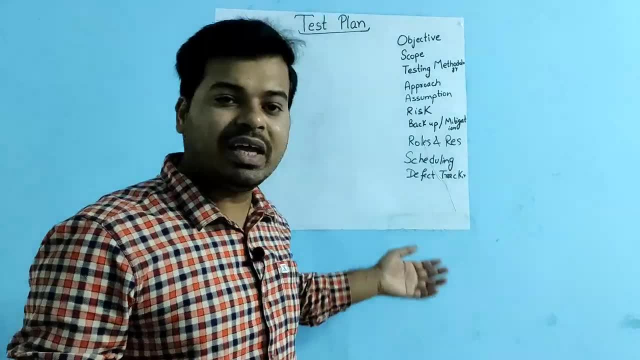 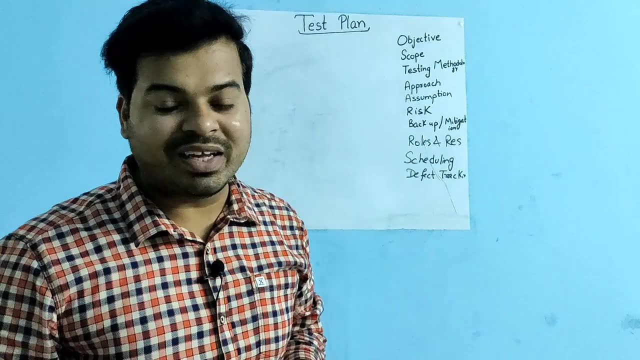 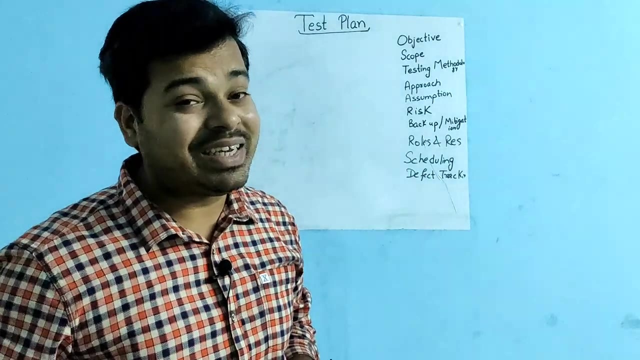 major, minor, severity and they will tell what is the priority types we are going to follow. so they can tell p0, p1, p2. i hope and whatever i'm talking is understandable by you guys. if not, link is there in the description: severity and priority. i have spoken in detail. please watch it and come to this video. so under 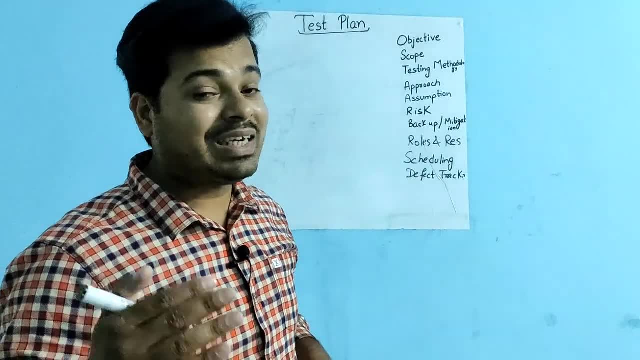 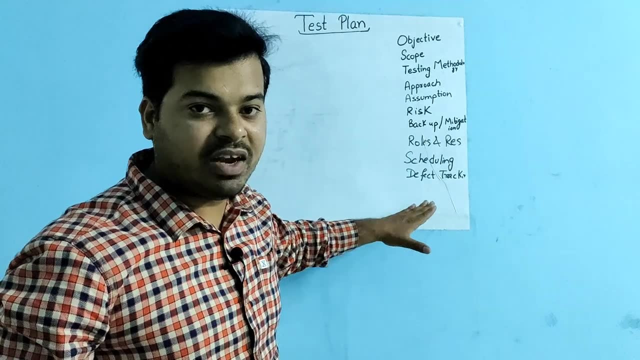 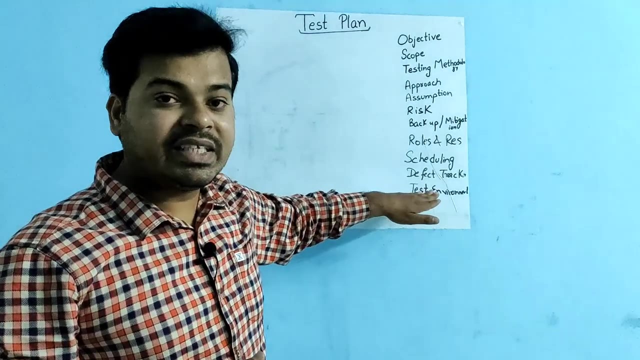 defect tracking. these four components will be there. let's move ahead to talk about the next component, next attribute: we have in test plan which is called as test environment. always remember, guys, test environment- the other names is called as test bed. it is the environment which my testing 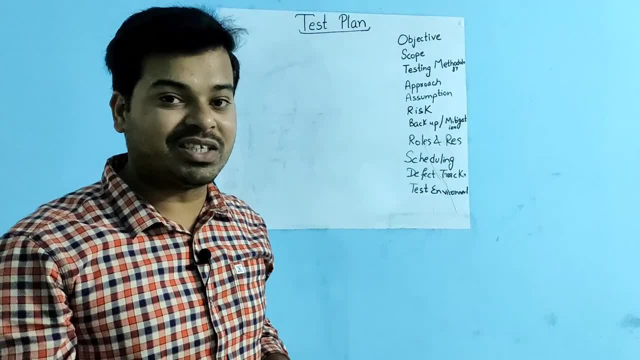 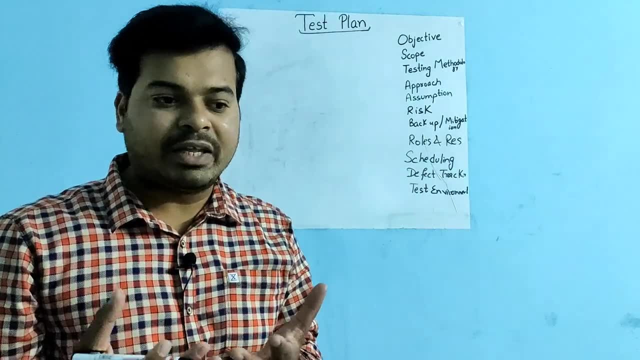 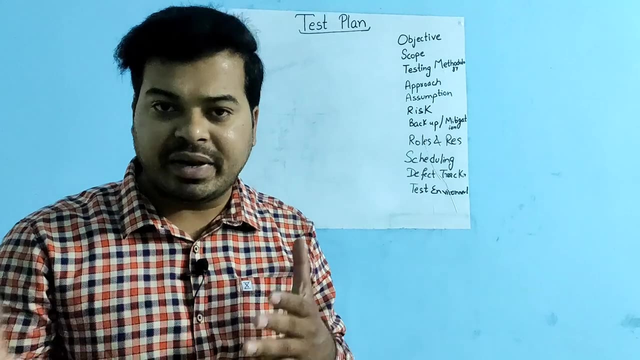 department people will use to test their application. so, under testing environment, while testing the application, what you know, things you expect that you should have to test it, the application, all those details will be written in this. let's say you are making a payment, so which credit card, debit card you need to use while making a payment? 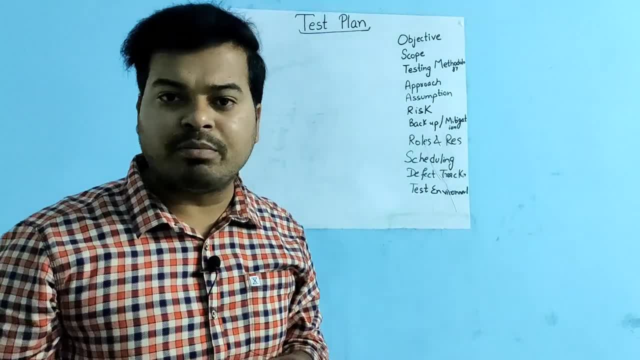 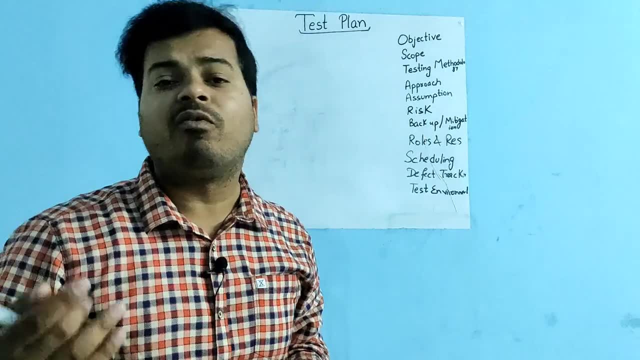 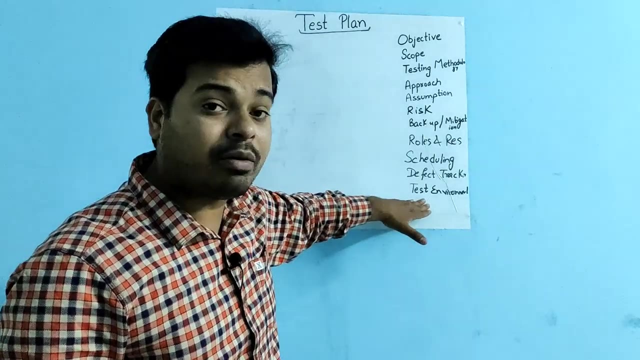 those details will be given here. in any company, there will be multiple wi-fi connected, so which wi-fi you have to use in order to use my testing environment. what is the test environment and what is the password of it- all those details which you needed to test the application in your testing environment. 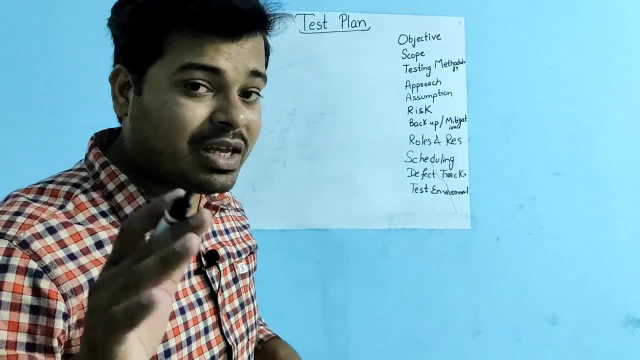 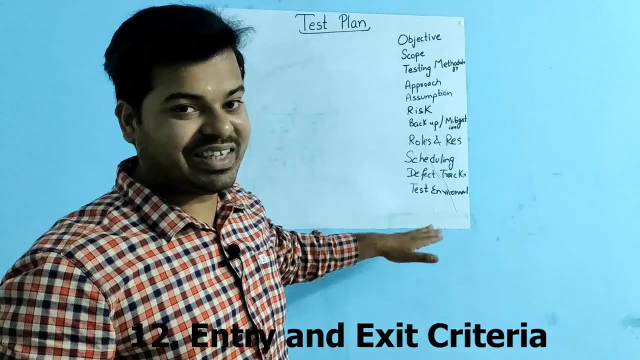 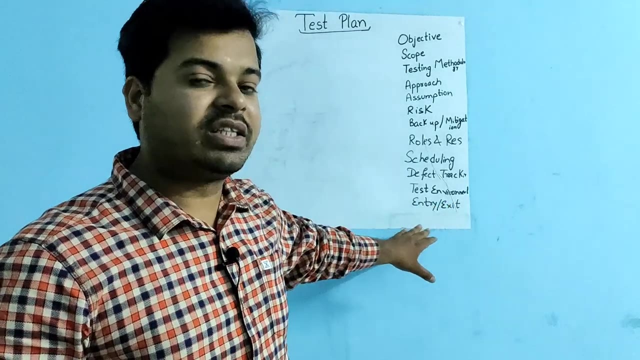 or your test bed will be written here. talking about, the next attribute we have in test plan is called as entry and exit criteria. now, talking about the entry and exit criteria, it is nothing worth. these are the set of condition that should be met in order to start any new kind of testing. 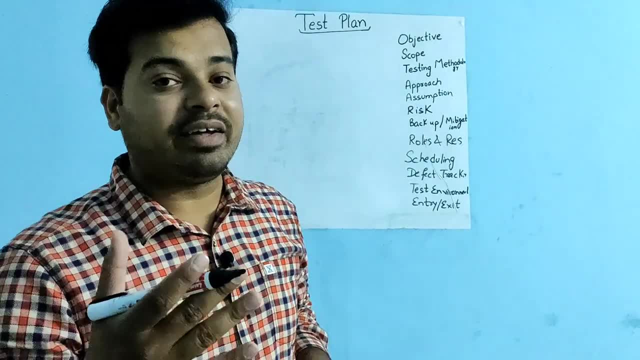 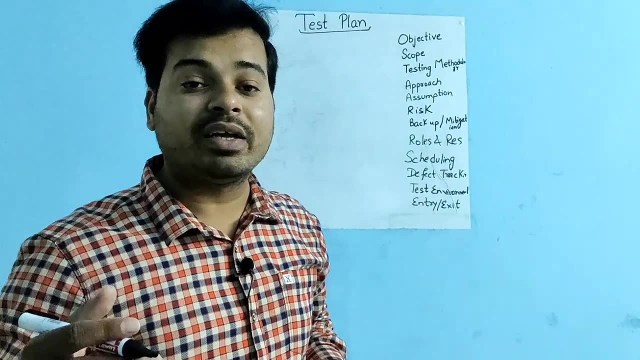 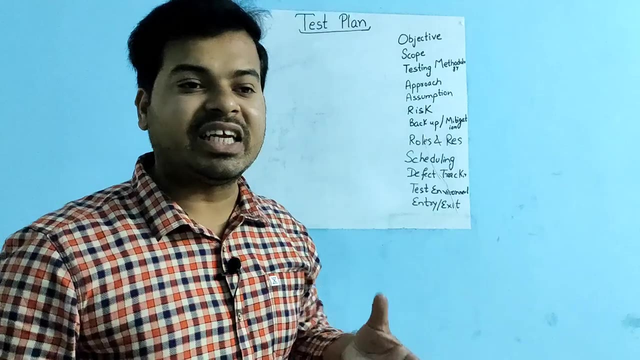 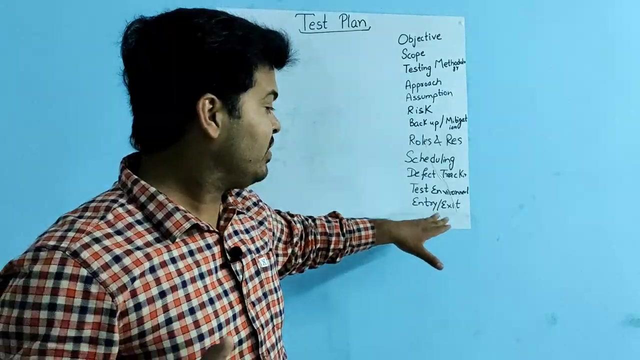 new type of testing and to end any any kind of testing. so these are the set of condition that should be made if you are doing any kind of testing and if you are trying to end any kind of testing. so these are the criteria that should match to start any kind of testing. so in SDLC software development lifecycle, every 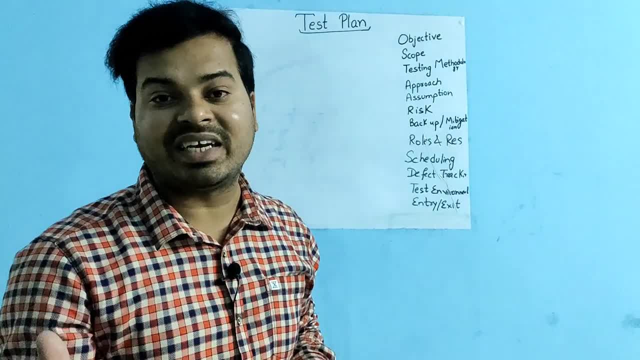 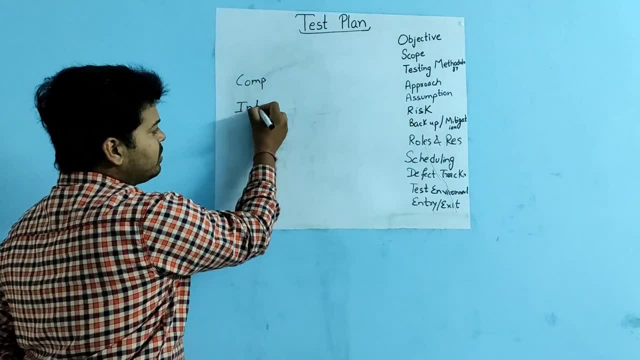 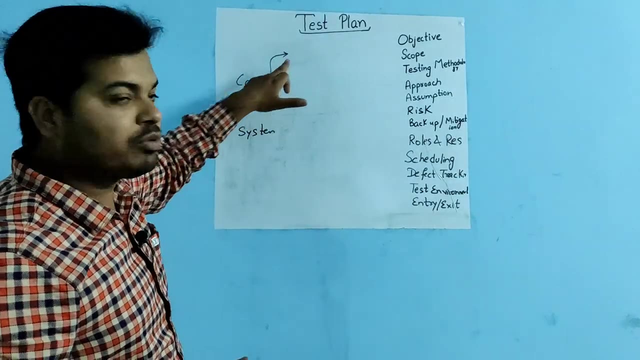 stages has got some entry and exit criteria. what are the major kind of testing you do is called as component testing, integration testing and system testing. when you are doing your component testing, what is the entry criteria to start your component testing? all those points will be written here. 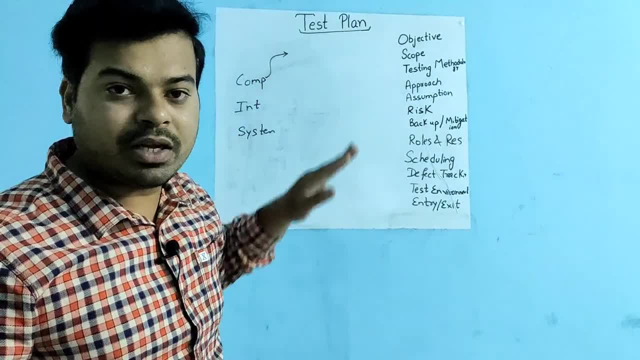 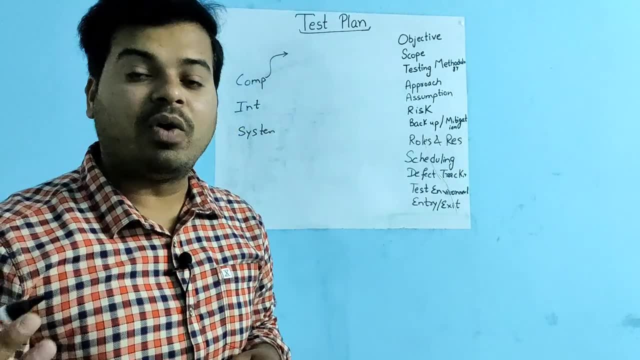 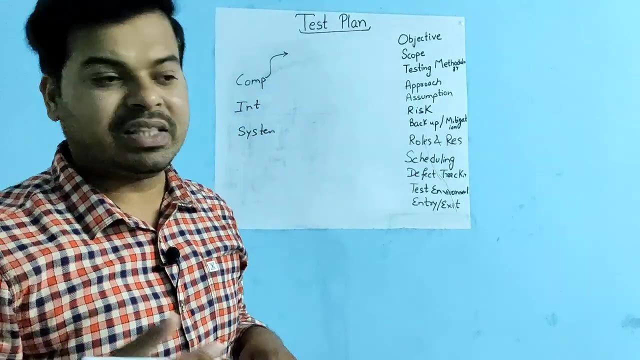 example, when you are starting your doing your component testing, the entry criteria is smoke testing or sanity testing should be completed. developer should give the build after doing white box testing. all the test cases should be written. my test cases should be approved by my test late. these are the some cases, some condition. 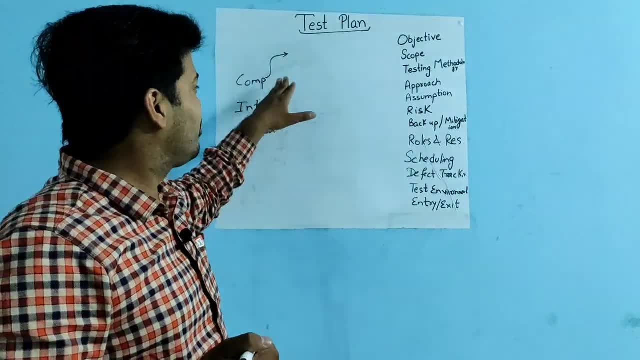 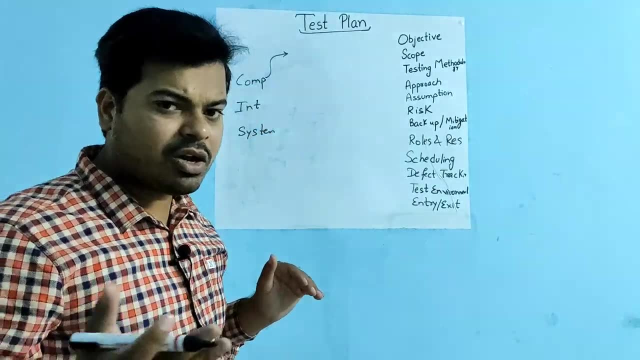 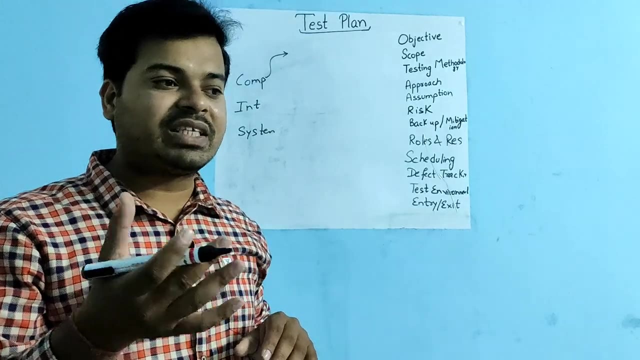 which should satisfy if I am proceeding with my component testing. so these are all. things are entry criteria, if you are going forward to the component testing. now let's talk about what. what is the exit criteria for component testing? talking about the exit criteria, I mean when you can say that oh, I have done my. 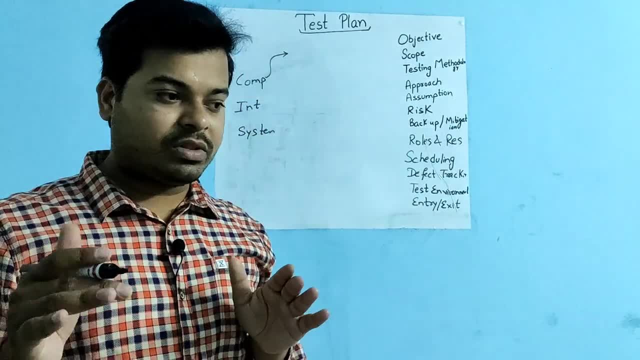 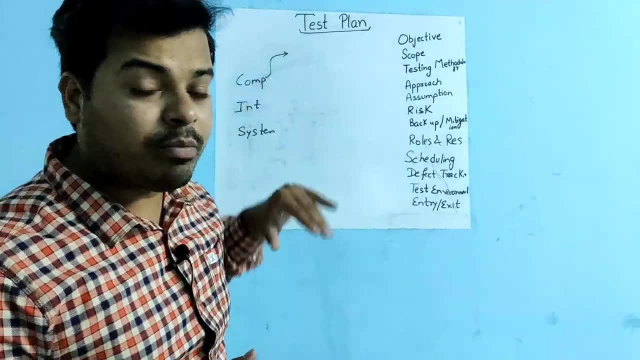 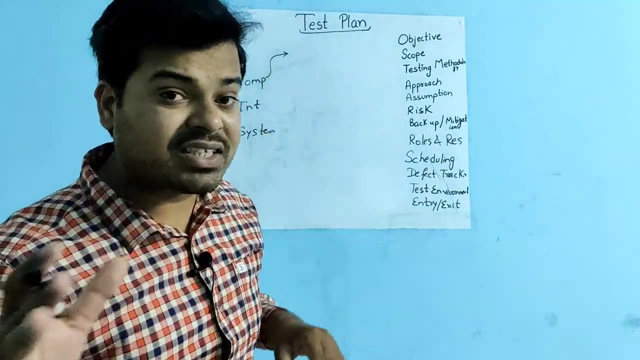 component testing fully. now I am proceeding with my integration testing, so this is whatever I'm going to talk- is not which every company follow, but this is the standard. so, talking about the exit criteria of component testing, it will be written like: 80% of the test cases should be passed. 80% of my component test cases should be passed. 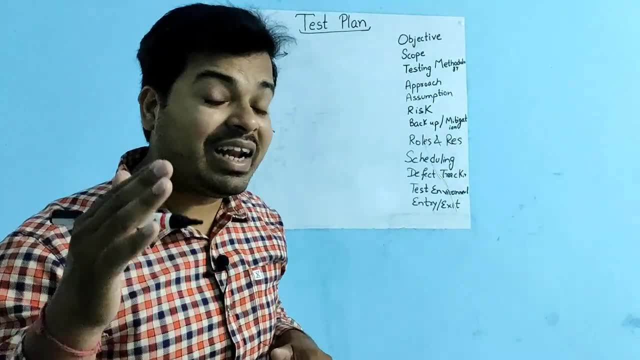 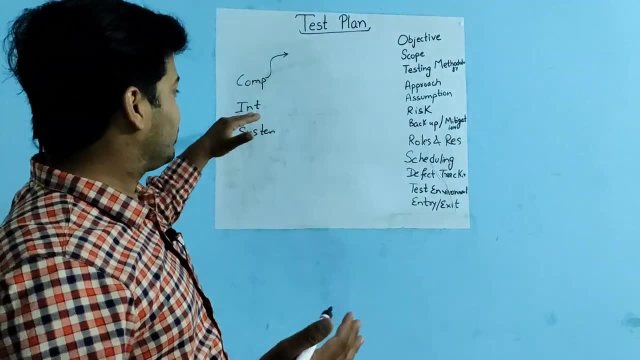 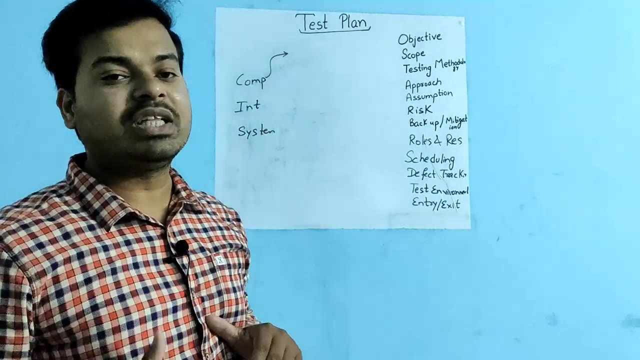 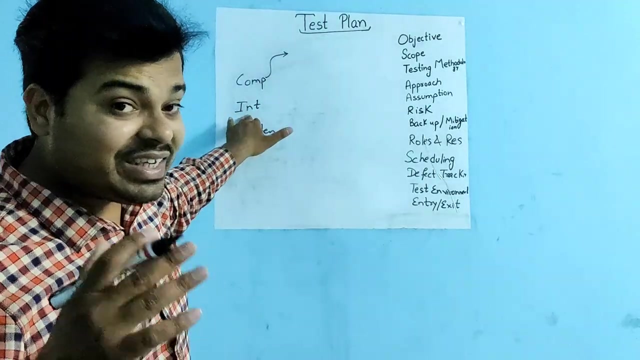 we cannot go to the integration testing until and unless there are more than two blocker severity defects. we cannot go to the integration testing until and unless there are five major severity defects. these are all. things are the exit criteria for my component testing. now let's talk about what are the entry. 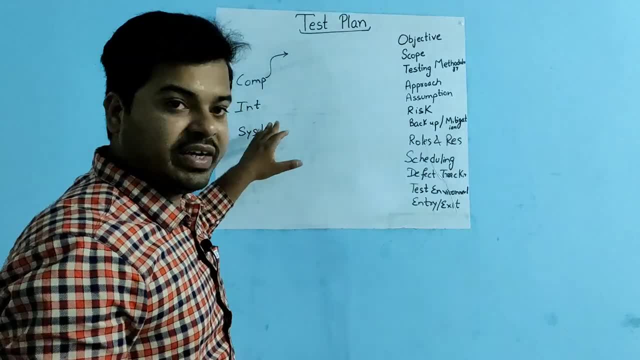 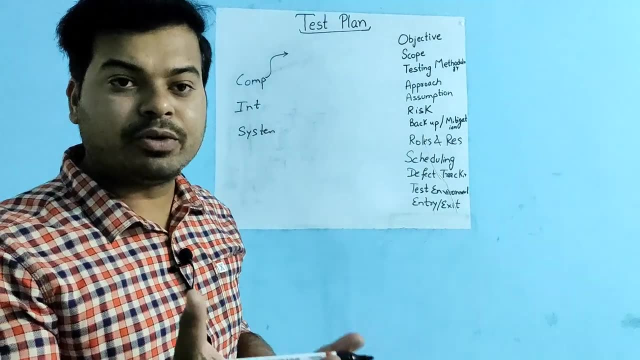 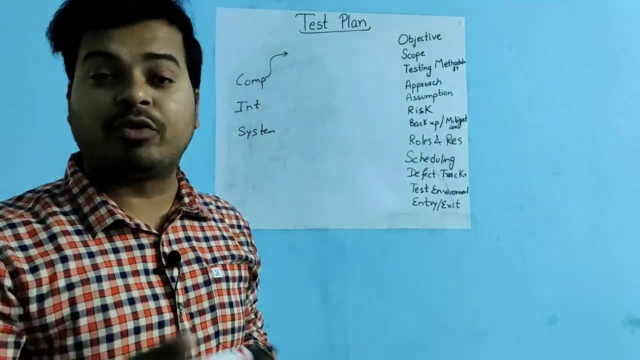 criteria for my integration testing. so entry criteria for my integration testing will be: it should make the exit criteria of my component testing, of my component testing. all the test scenario, all the integration test scenario should be written. all the integration test scenario will should be approved. developer should have done the white box testing then. 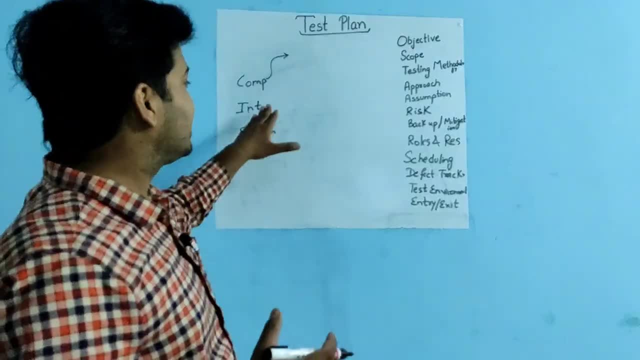 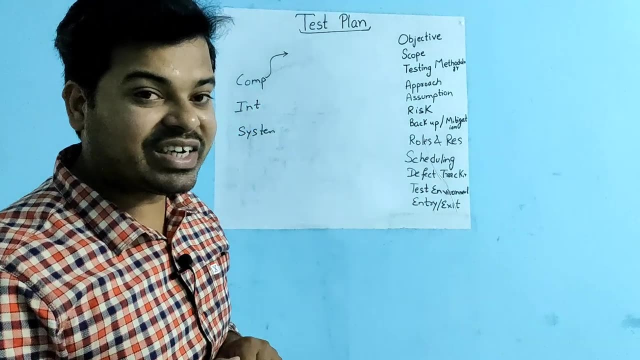 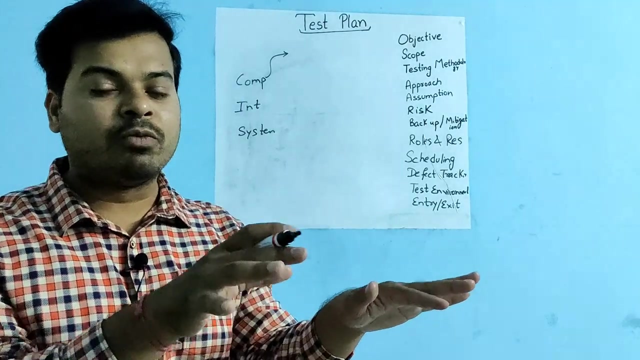 he would have given the build to us. those are all. things are the entry criteria for my integration testing. now let's talk about what are the exit criteria for my integration testing. exit criteria for my integration testing, it means when you can say that my integration scenarios, everything is done and now I'm moving towards my system testing so you can go ahead. the system testing only after exit criteria of integration is satisfied. so what is that? so, under my exit criteria of integration testing, I will say that we cannot go to the system testing until and unless there are more than five critical severity bugs present, we cannot go to the system testing. 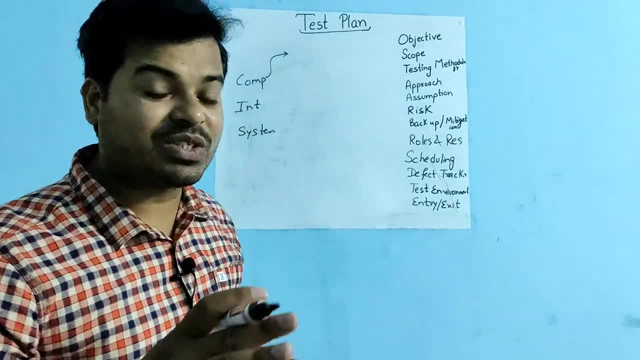 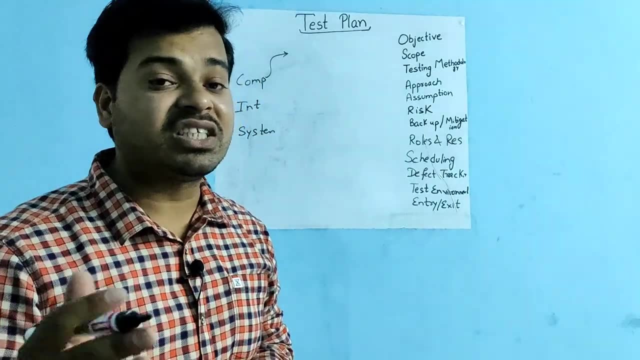 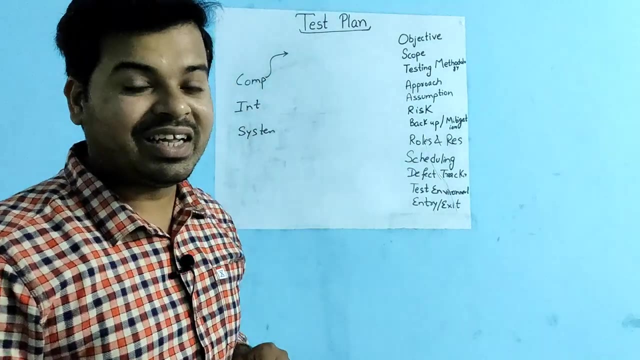 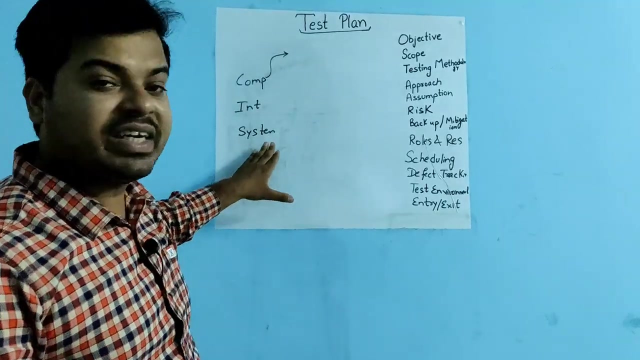 until and unless 90% of my integration scenarios are passed, we cannot go to the system testing. there are more than 10 major severity bugs present, so these are all are the exit criteria for my integration testing. now let's talk about what are the entry criteria for my system testing. so, talking about the entry criteria of my 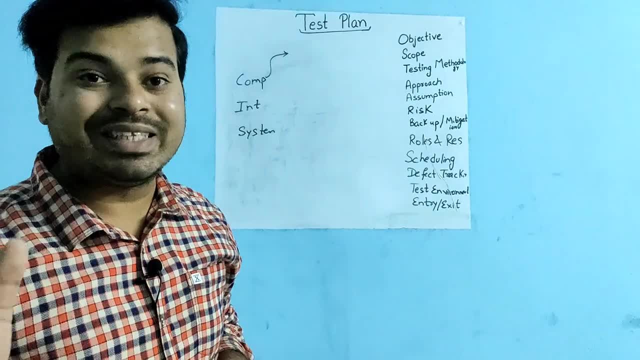 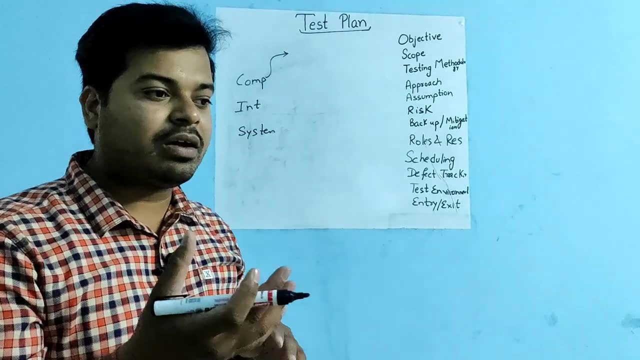 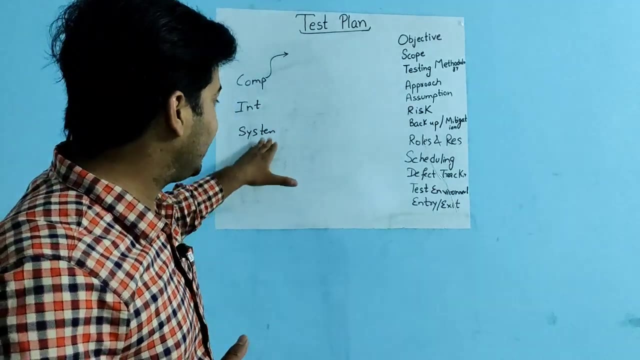 system testing. the first point will be: it should meet the exit criteria of my integration testing and most of the module should be present to test the system behavior of the any application. so these are all the entry criteria of my system testing. now what will be the exit criteria of my system testing in exit? 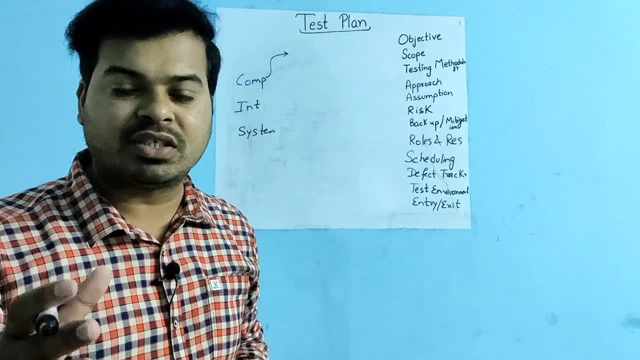 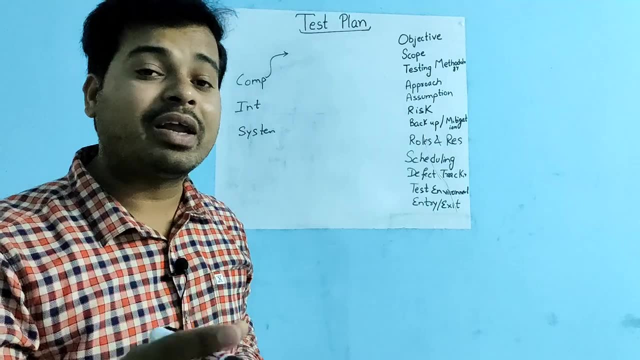 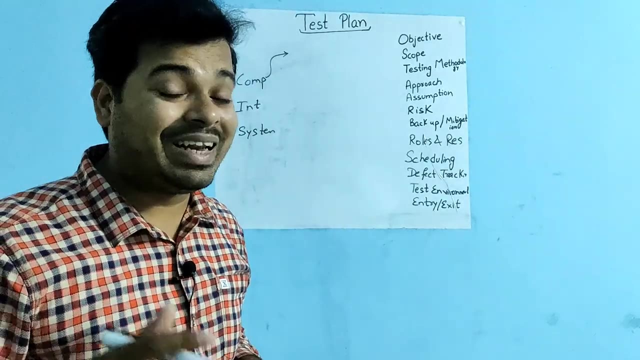 criteria of my system testing, I will say that 99% or 100% test cases should be passed. there should not be a single blocker or critical severity bugs present. so these are all are the exit criteria of my system testing. let's go ahead to talk about the next. 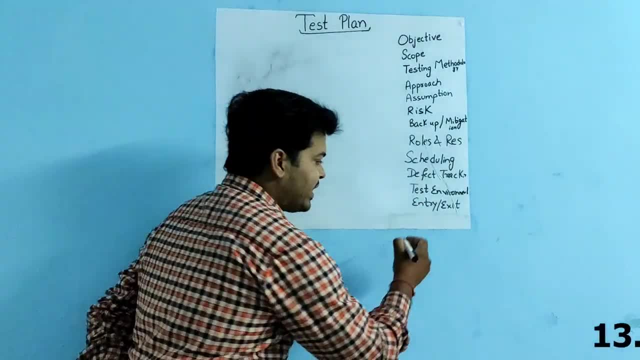 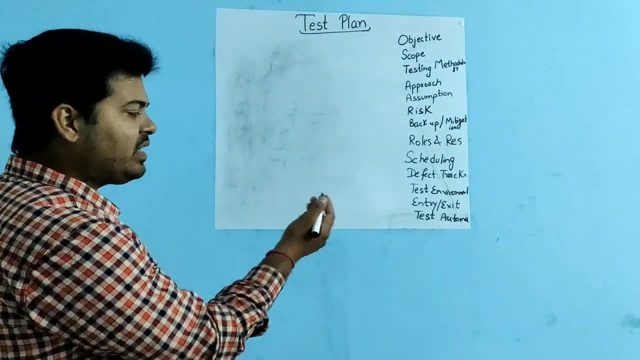 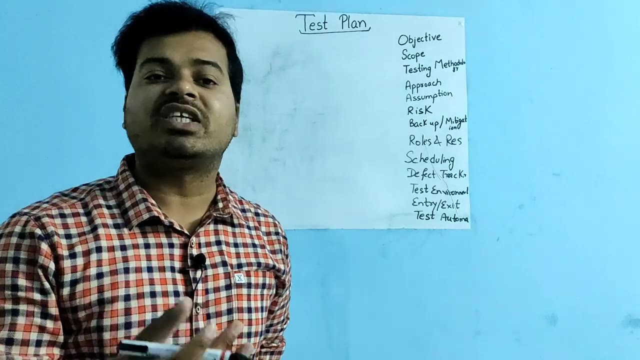 attribute we have in test plan that is called as test automation. so when you are writing test plan and you are writing the attribute of test automation in test automation, you will be having plenty of things like: which, in all features are to be automated, those names which, in all feature, are not to be automated, which. 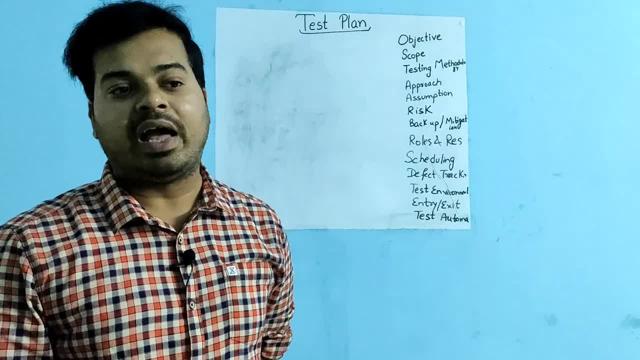 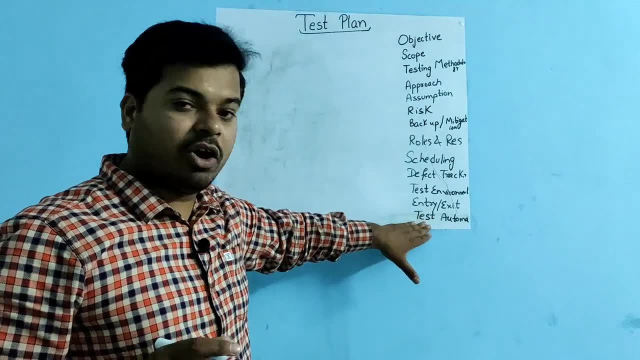 tool I am going to use as a part of my automation and which framework I am going to use as a part of my automation. so these are all. things are the part of test automation. so the next attribute we have as a part of test plan is called as: 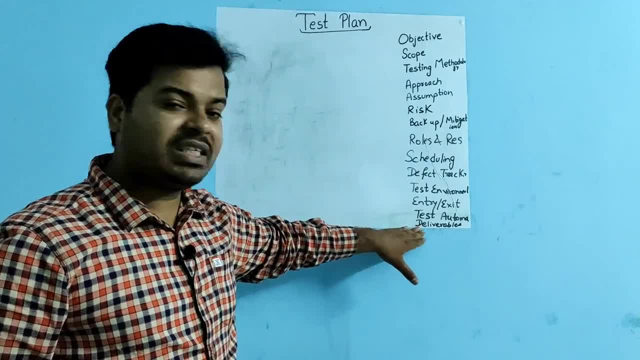 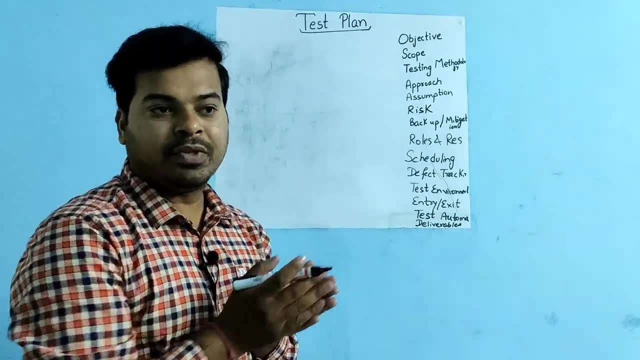 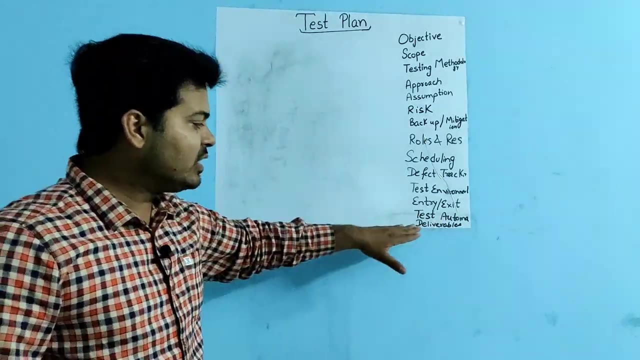 deliverables. so deliverables are nothing, but these are the outcome from my testing team, which is what I am going to give it to the customer. so what are the things my testing team will give it to me? and, finally, we are going to give it to the customer example. so in this, multiple things will be written: test. 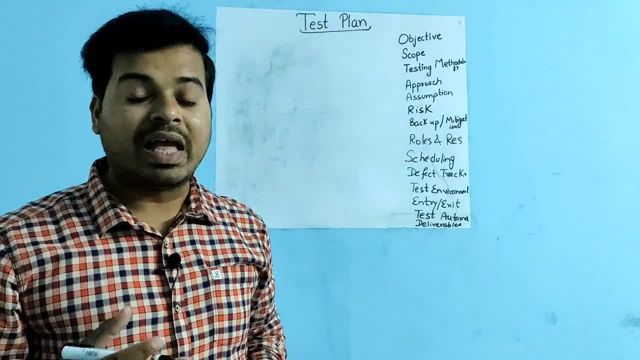 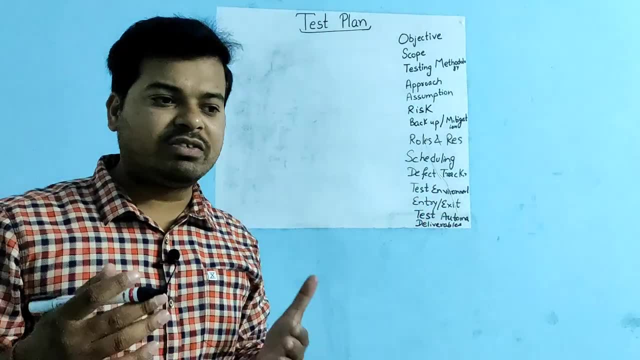 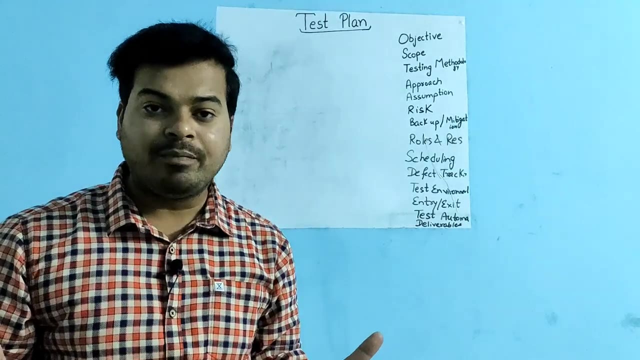 cases, test scenarios, traceability metrics, execution reports and also the test report, defect report, release notes. so those are not the deliverables which will give it to the customer at the end of the project, when testing is, testing is completed and finally, we are going to give it, give the software to the